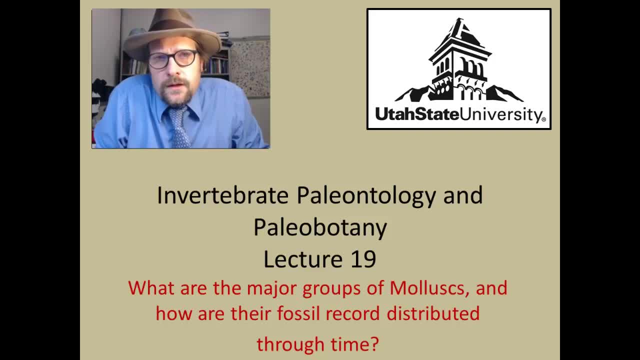 outdiversified by the Anthropods, including the insects, But in many ways, when you look at the numbers of species, the mollusks are much better represented in the fossil record. Mollusks include slugs and snails, scallops, clams, oysters and cephalopods that include 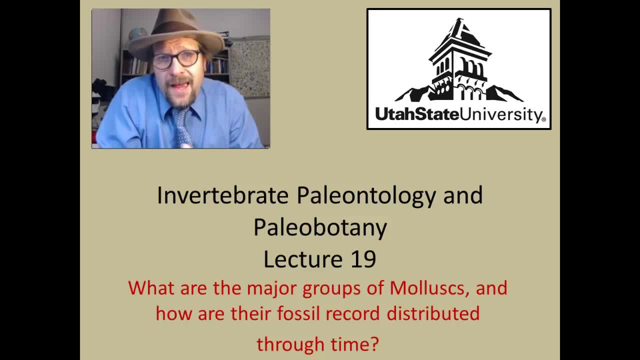 squids, octopuses, as well as ammonites and bulimonites. It is a really big group of animals to cover in a single lecture, But we can simplify the group when we look at the archetype of mollusca or the shared 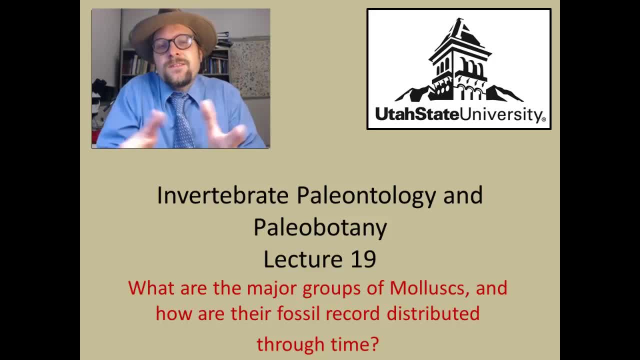 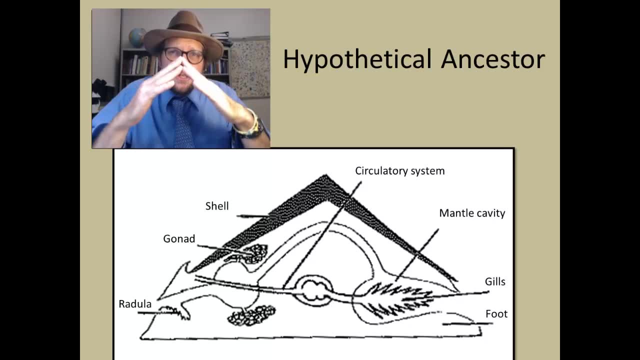 features that all of these groups have in common, or at least ancestrally they have in common. Here it is. It is a rather weird looking animal. It has a cap-like shell composed of calcium carbonate on top, which is secreted by a layer of tissue below called a mantle. It has a 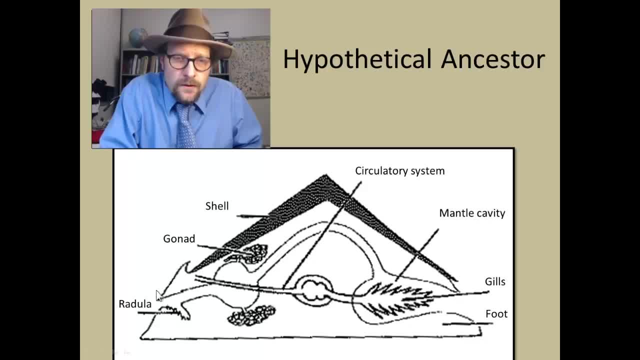 gut. It has a mouth at one end and an anus on the other end. It poops into a chamber called the mantle cavity. It contains a gill. Gills are found in all mollusks except for land snails, which develop lungs. 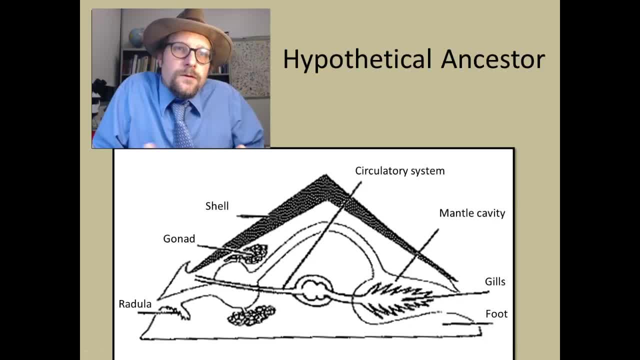 Gills are an important adaptation because it allows for respiration to more easily take place in the body. Cells along the gills can take up oxygen from the water and transport this oxygen throughout the body to the canal system system of a primitive circulatory system. 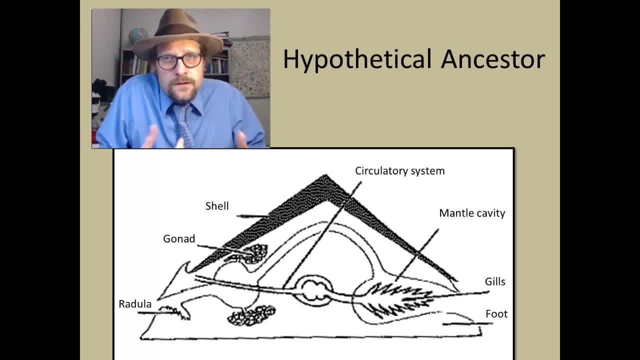 The reason oxygen is needed is that it is required in cell mitochondria to be used in the production of ATP molecules that help produce the energy needed for cell growth. Cells can produce ATP without oxygen, but this only produces a small amount of ATP, hence only used for short periods. 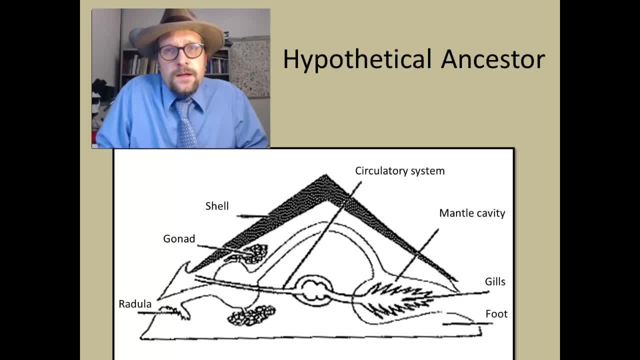 Having a mechanism to bring oxygen into the cells of a body is important, especially since many mollusks cover their bodies with hard shells and hence it is difficult to gather oxygen out of the surrounding water, so they have developed gills. Brachiopods do not have gill structures because they have the lofophore, in which, in addition, 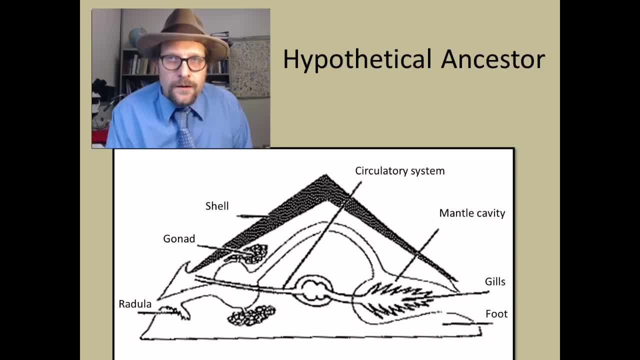 to gathering food, particles can also gather oxygen from the water. Mollusks do not have a lofophore. Food gathering in mollusks is really different. They have a simplified mouth that sometimes has teeth called the radula. This means that mollusks can pursue food sources and many are mobile, some as grazers, others 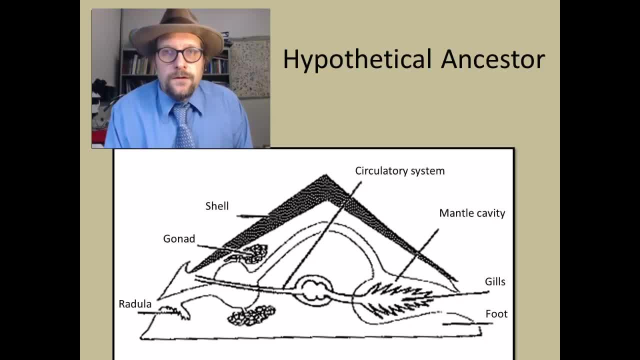 as active predators and even some filter feeders. The lack of a lofophore suggests that mollusks are more distantly related to brachiopods and likely arose from a food source. The lack of a lofophore suggests that mollusks are more distantly related to brachiopods and likely arose from a food source. 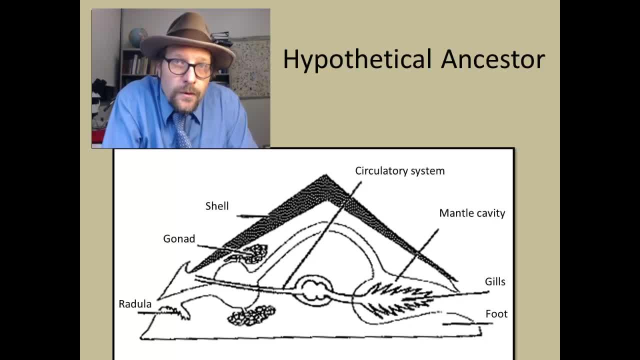 The lack of a lofophore suggests that mollusks are more distantly related to brachiopods and likely arose from a food source. The foot projects out the very back of the organism, And this foot provides a method to crawl around on the surface of the ocean floor. 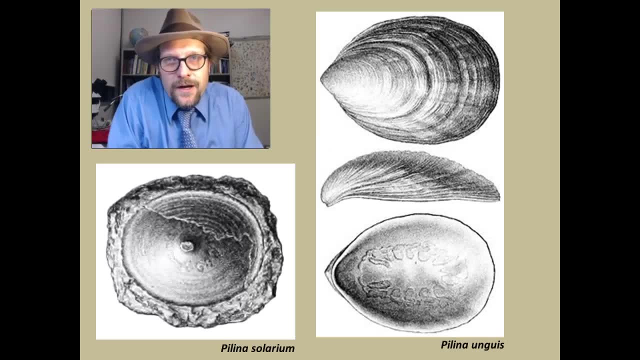 This hypothetical ancestor is represented in a fossil record with a group of early primitive mollusks called Monoplac osobyh reh. Monoplaceyap. reference looks like this: One of the well-known primitive members is the genus Pellinia from the Silurian of Northern. 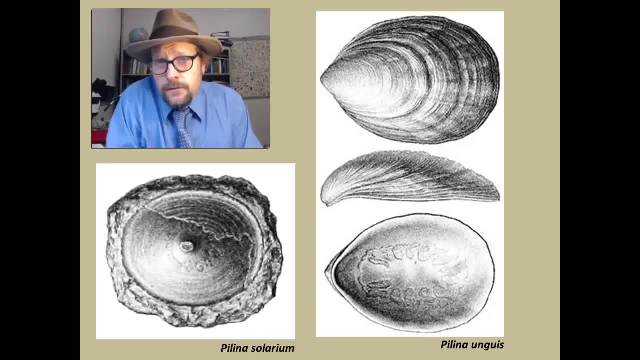 Europe. Pellinia has a single top shell, has muscle scars indicating that it lived on the ocean floor and crawled around in the mud and was protected by this hard shell from predators that would eat it. For many years, the Monoplactifora was thought to be an extinct group of mollusks, having 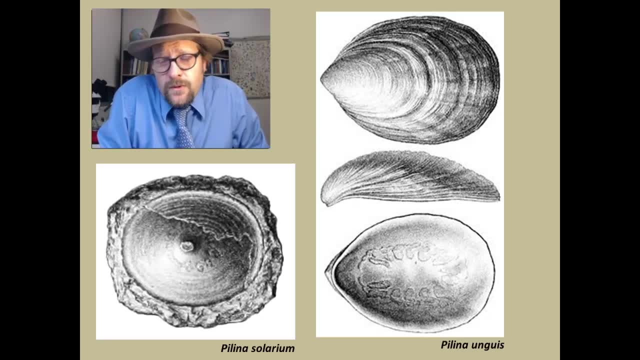 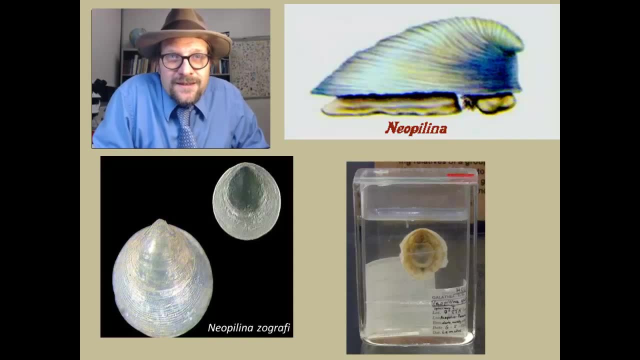 perished sometime during the late Silurian, with a fossil record from Cambrian to Silurian. But in 1952 scientists discovered a living member called Neopellinia from dredging the deep ocean floor. This was a really important discovery because it allows us to study a very primitive group. 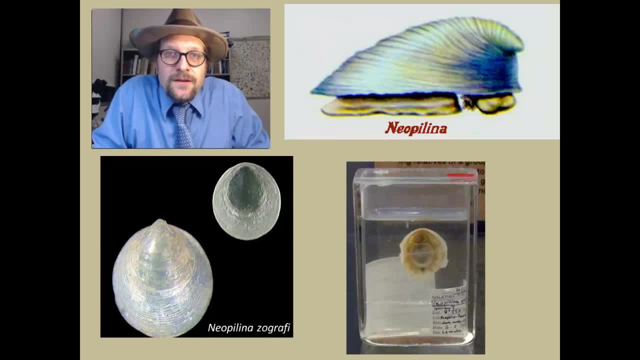 of mollusks. One discovery was that Neopellia has a circle of gill structures around the outer part of the mantle. with a central foot It crawls around the ocean floor eating food that it finds with its mouth, much like a 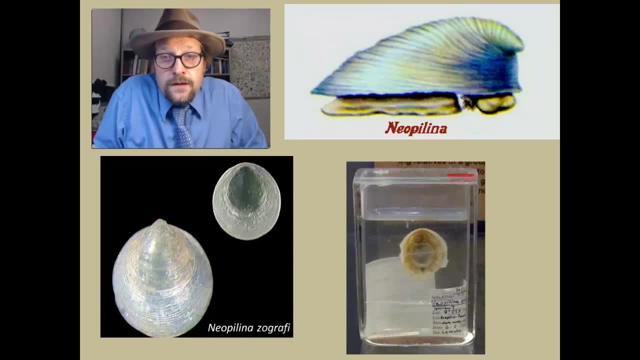 snail does. One interesting realization was that Neopellia was segmented, meaning that it had a series of gills and muscles, and this suggests that Neopellia and all other mollusks are closely related to Annelid worms. 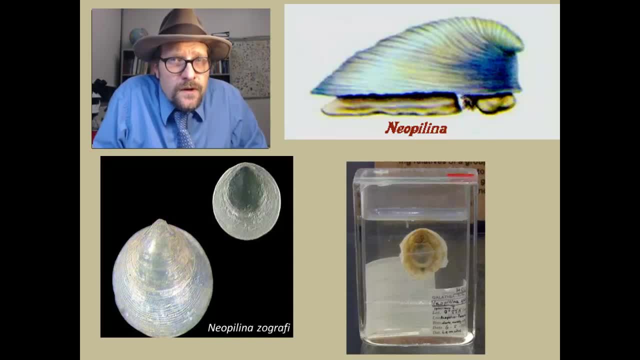 Annelid worms are a group that includes earthworms, Airworms with segmented bodies, Molecular analysis of mollusks and living Annelid worms support a close relationship between these two groups. Sadly, we will not be talking much about the fossil record of Annelid worms because, beside 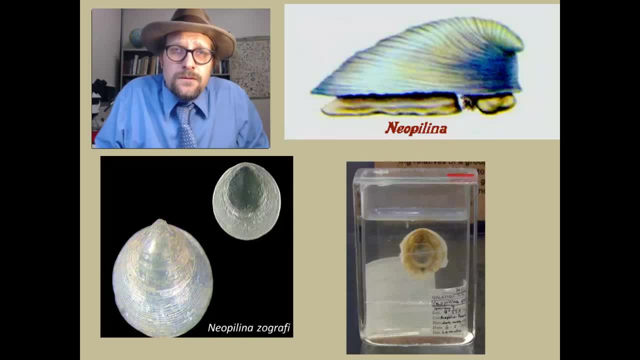 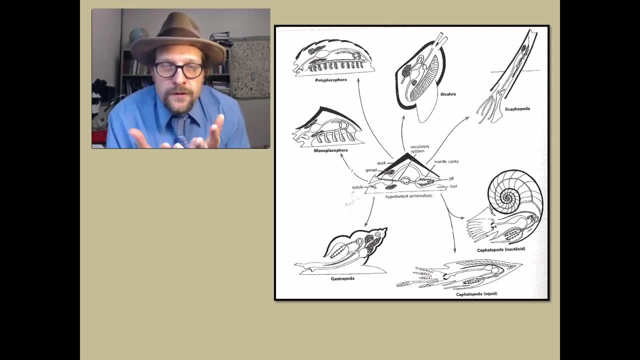 trace fossils. there is not much of a fossil record of these guys. From this primitive body plan we can envision ways in which the various groups of mollusks arose. Annelid worms could become segmented, like in chitons, paired like in bivalvia, or elongated. 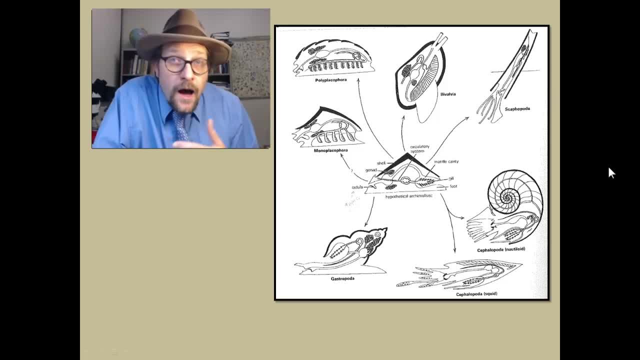 into tubes, like the scaphopodids, or coiled, such as in gastropods, and cephalopods such as nanoloids, or even internal, like in squids. Note that the shell can also be lost in many groups, like slugs, that we will talk about. 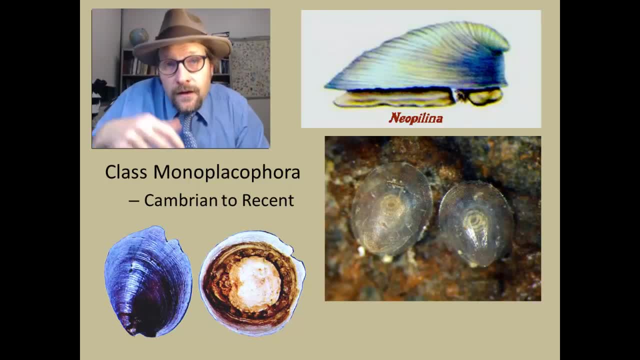 Now let's look at each of these classes within the phylum Mollusca. Now, there are seven major groups or classes. The first group is the Monplacophora, which are considered the most primitive group. Most fossils are known from the Silurian and Ordovician, but with a surprisingly sparse. 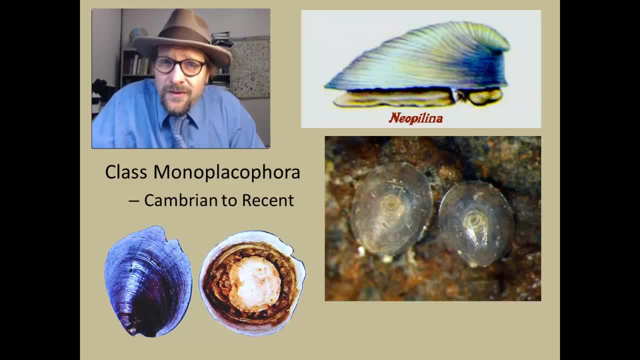 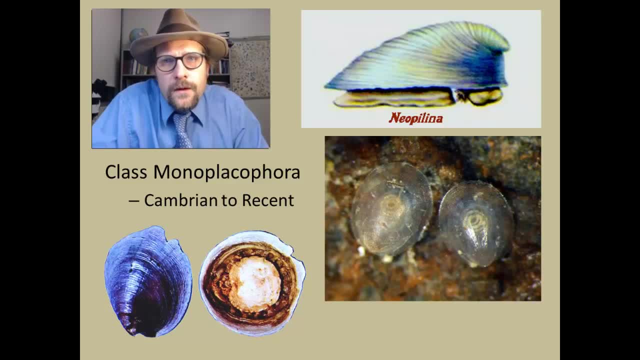 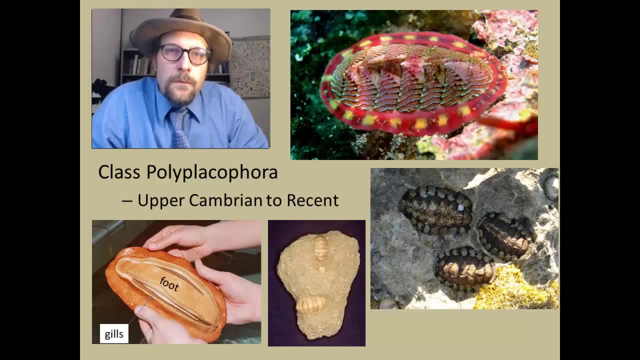 This means that the group was never diversified. The group is either diverse or widespread throughout. most of the Mesozoic or Cenozoic or the habitats that they occupy were not ideal for fossil preservation. Now the next group is the class Polyplacophora, which includes the chitons. 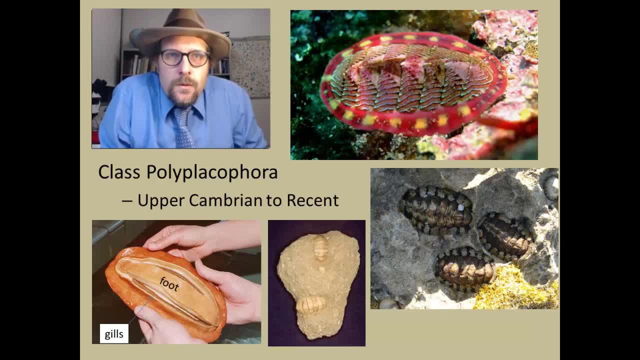 They are flat, oval-shaped mollusks with 8 overlapping dorsal shell plates or valves, bordered by a thick girdle forming the mantle that can be covered with hairs or spines. They kind of resemble- to me, at least- roly-poly bugs. 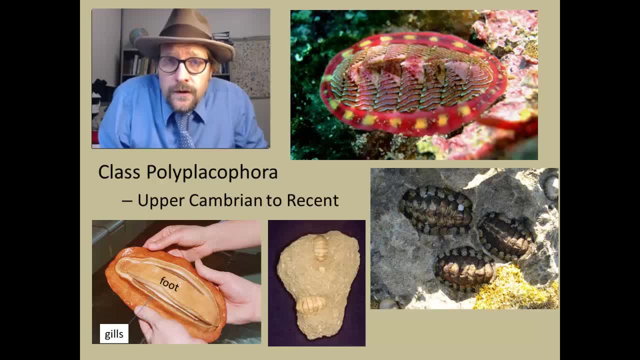 The mantle cavity contains multiple pairs of small gills surrounding the foot, with which the animal typically clings to hard surfaces. just like the monoplacophora, The plates can be reduced, or even internal in a few species, such that they can have 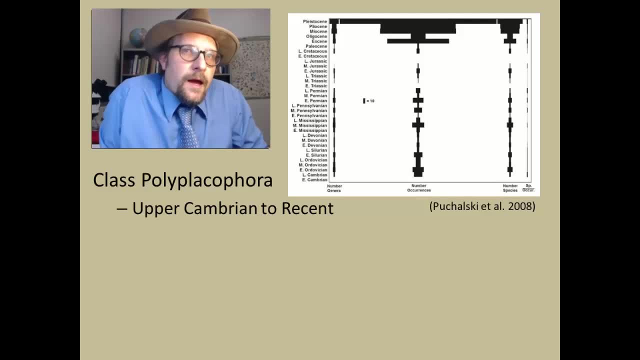 a worm-like body. The fossil record of the Polyplactophora is mostly late Cenozoic, with a number of occurrences dating back to the early Cambrian. They are not particularly well represented in the Mesozoic and only a few forms are. 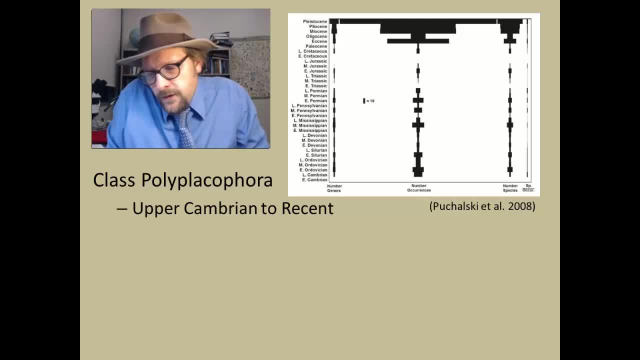 known during the Triassic, During the Oligocene, onwards to the Pleistocene. they are much better represented in the fossil record. Many are small, but some forms got to be over 10 cm in length. The next group is the Scaphidophora. 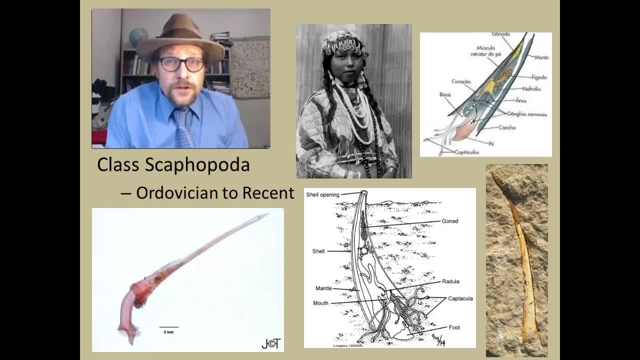 The tusk shells, known from the Ordovician to the modern. These are really unusual creatures that make their living burrowing down into deep marine muds. The mouth opens below as a foot digs down with a capitellium, a tentacle-like appendage. 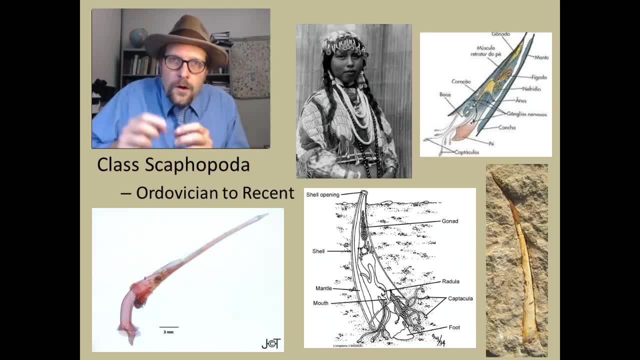 that brings food to the mouth. The anus opens at the narrow opening at the top of the horn shell- Two openings. These are common fossils and here in northeastern Utah I found them in the late Permian Park City formation. Because of the shape of the shell, with the two openings on either end, the modern tusk. 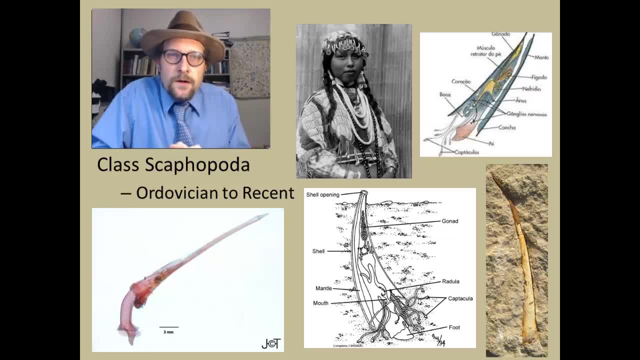 shells were adopted as the currency in California, where the modern genus Deltalium was used to trade for goods. The shells were also used among early Americans along the Pacific coast as decoration and a sign of wealth and prosperity. These shells are really rare and made a good currency to various tribes along the 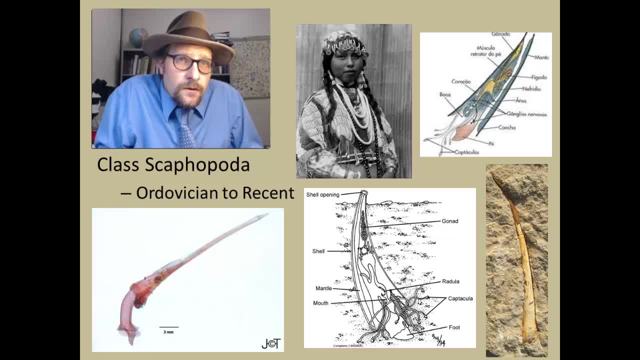 western coast. Shells were also used along the Atlantic coastline for currency, but came from a different group, the bivalves, which had to be manufactured by local tribes, since they didn't have two holes on either end, so they had to drill a hole through to make these beads. 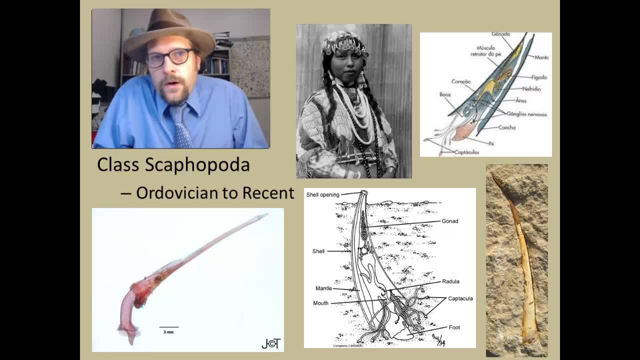 Those other beads are the ones that formed the wampa currency, that were used by the native tribes of the Iroquois Confederacy and the Algoquintin tribes. This was abandoned when Dutch colonists developed an easy way of manufacturing these shells. 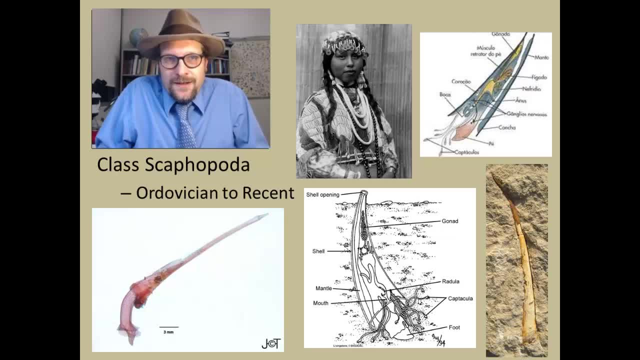 and basically flooded the market with cheaper beads and causing a huge amount of inflation. This, of course, resulted in the later adoption of a gold standard for trading for goods. We still use the term shelling out in reference to paying for something, and that harks back. 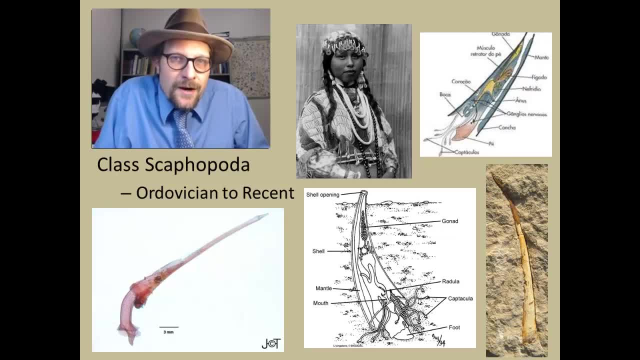 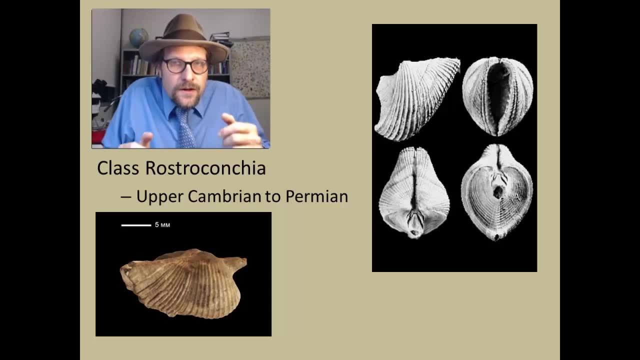 to the use of these shells. The next group is the only class of mollusks that are entirely extinct. These are the Rostecontia. Despite having two valves, the Rostecontians secondarily developed two valves. Larval forms lack a secondary valve and they somewhat resemble the primitive monoplactiforians. 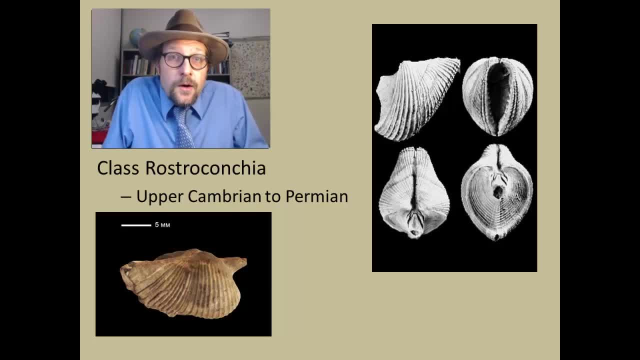 They were recognized as a separate class in 1916. They are particularly diverse during the Ordovician, with about 400 known species. Each shell enclosed an internal anatomy that included a mouth on one side and anus on the other side, with lateral gills and a molluscan foot. 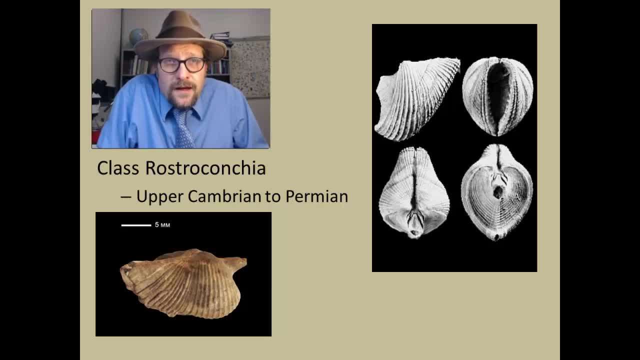 They have a shell that has a long pipe that served as the anus exit and in some ways resemble the Tufts shells, the Scapapoda, which they may have given rise to. They fed on a variety of animals. They fed on the ocean floor, with most forms buried in the sediment. 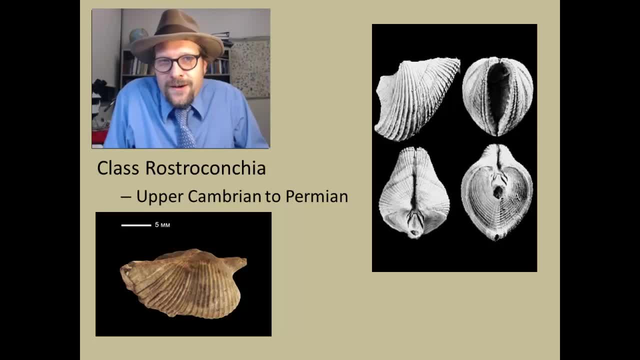 They diversified during the Ordovician, but hung on the fossil record during the late Paleozoic, becoming extinct at the Permian-Triassic boundary. Mollusks are great survivors, but even the greatest extinctions on Earth took out some. 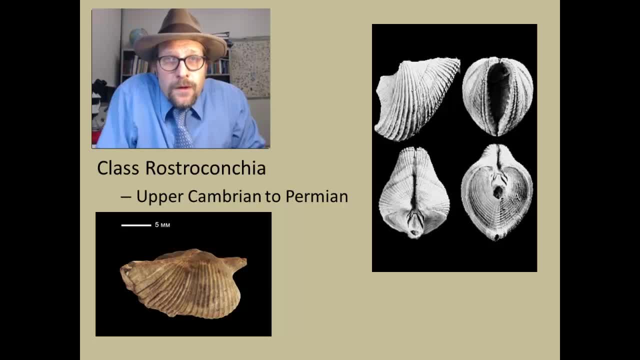 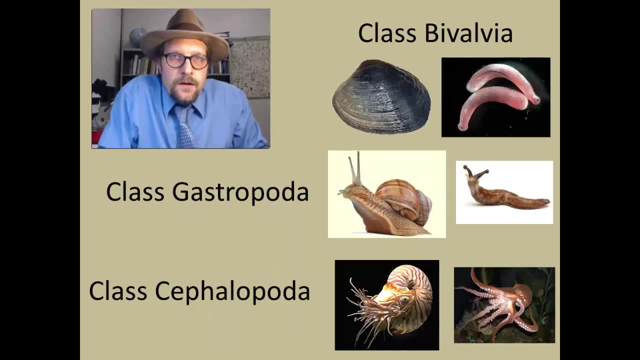 of these groups. However, the big three classes of mollusca survived this extinction with a remarkable fossil record: 1. Bivalvia, 2. Gastropoda, 3. Cephalopoda. The three classes of mollusca are the bivalvia, the gastropoda and the cephalopoda. 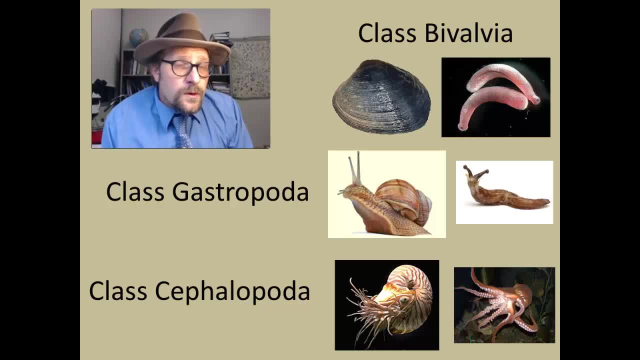 Each of these are very diverse. They also include shell-less forms: For bivalvia, we have the shell-less and placophora. For gastropods, we have the shell-less slugs, which are a polyphyletic grouping. as many 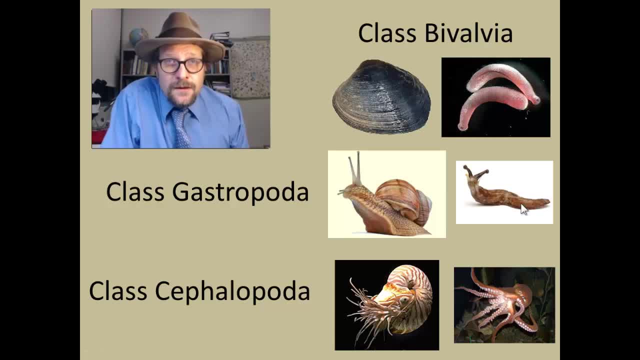 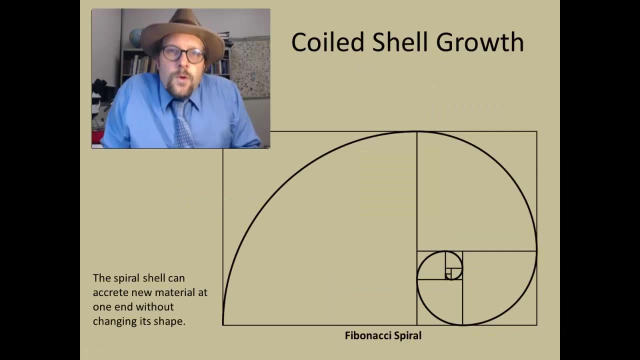 gastropods have lost their shells. 4. Snails. 5. Plumeneat slugs. 6. Cephalopoda. The cephalopoda includes the shell-less octopuses. For our class, we will talk mostly about the forms that have shells. 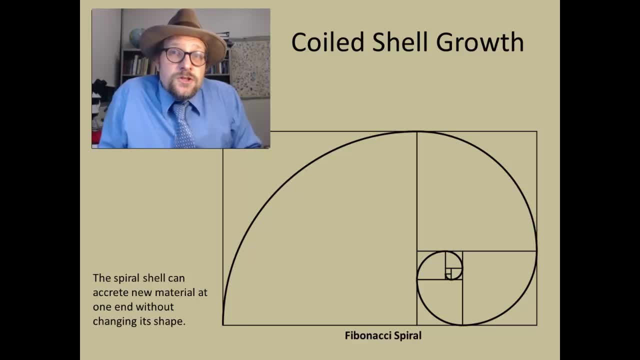 The morphology of the shells in these three major classes share the trait that they grow through the Fibonacci series or through other logarithmic scales in which, as the animal grows, it retains the same proportions. Hence, each sequence of growth must be functional, be functional and isomeric growth. 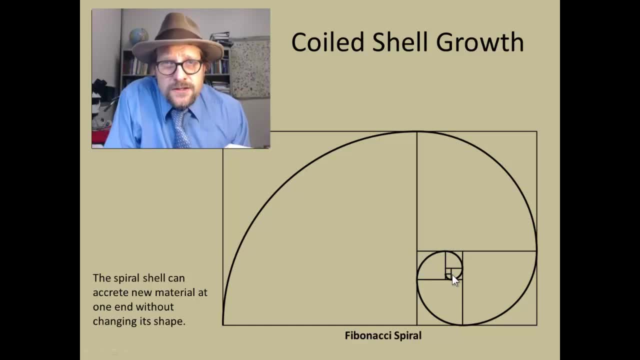 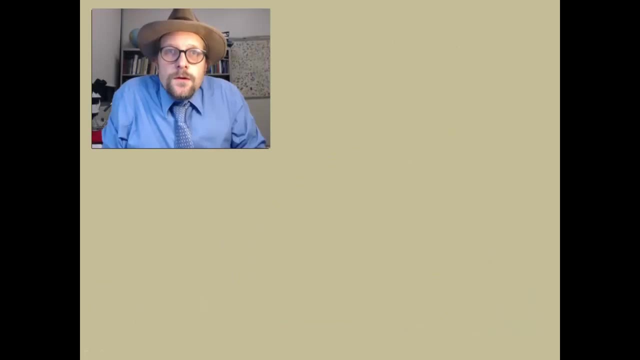 So notice in this picture here that each box shows a shell with the same dimensions as the following box, such that with each new growth the shell resembles the same form as before, but has only been scaled up to a larger size. Using computers, researchers can play with the theoretical limits of such coiling and 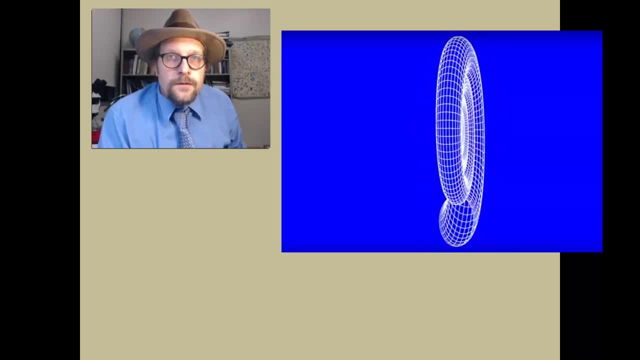 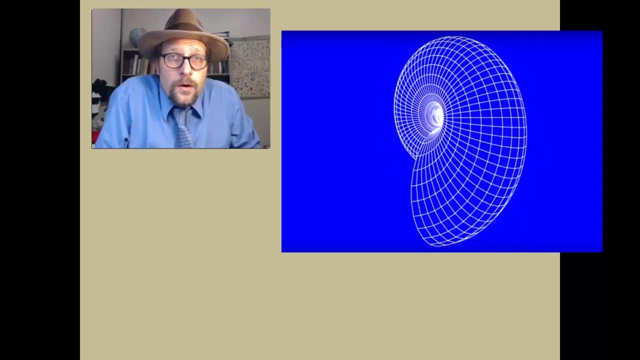 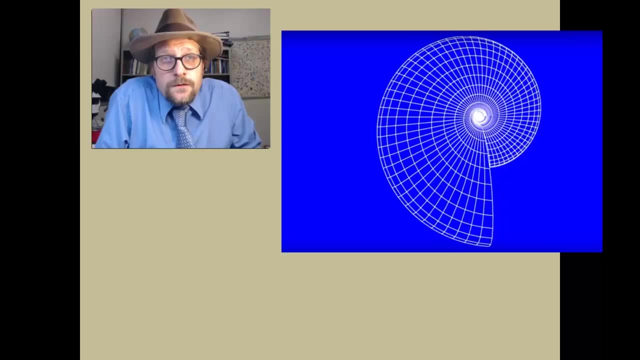 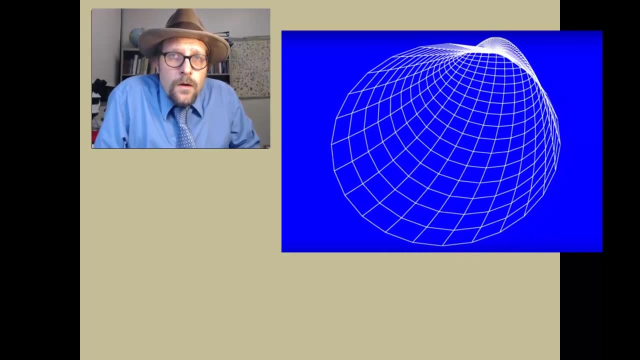 use various simple growth parameters to build models of different growth patterns. Moving from the coiled shells found in some pleuroorbid gasteropods, you can change the rate of growth to produce the coiled shells found in some nataloid cephalopods. 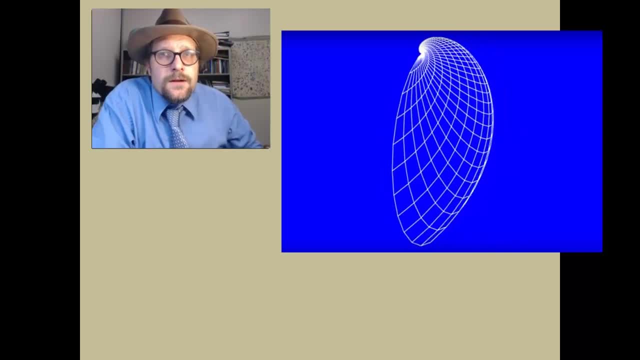 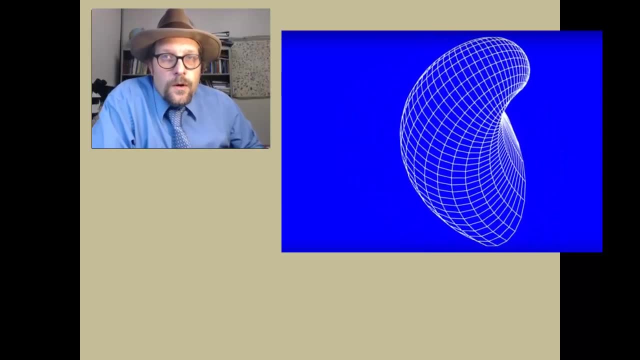 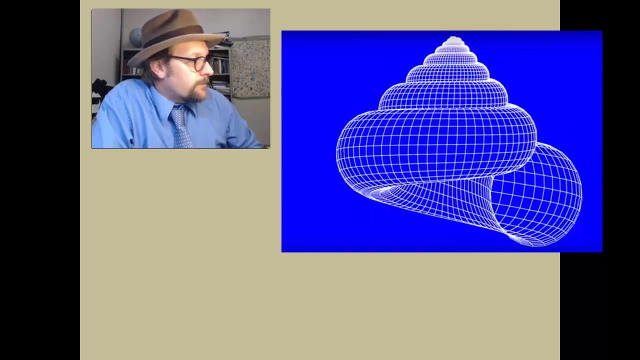 Or you can reduce down to the uncoiled shell in many bivalves, which have shells that are uncoiled, or twisting the growth around the axis to produce a shell that resembles a gastropod, a snail shell. 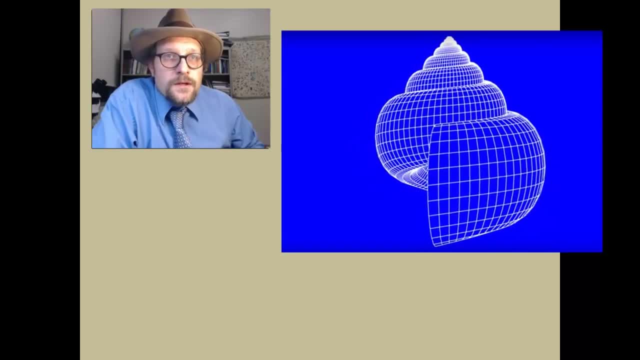 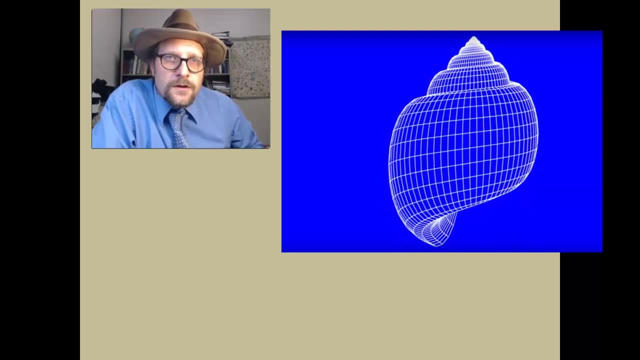 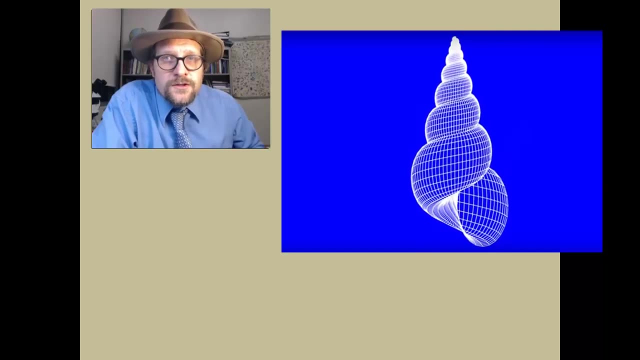 Of course, playing with these parameters can produce any combination of whirls and twists in the shell that you can build a complex range of experimental morphologies and, using a few parameters, explain a whole range of shell morphologies observed in the fossil record. 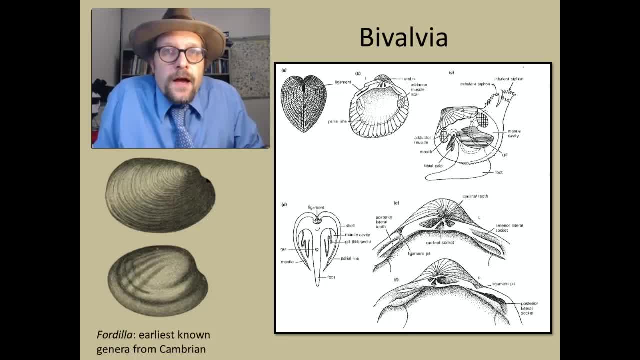 Let's look at the bivalvia, the first class of the big three mollusk groups. The oldest member of the group is Phorodinia from the early Cambrian. It closely resembles modern bivalves, indicating that the group has remained remarkably conservative. 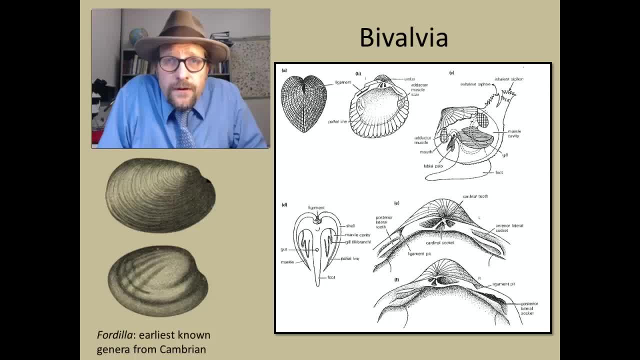 throughout the Phanerozoic. As their name suggests, bivalvia have two valves or shells. Unlike brachiopods, the bivalvia have shells that are held together by a stiff ligament rather than contacting each other with a complex hinge. 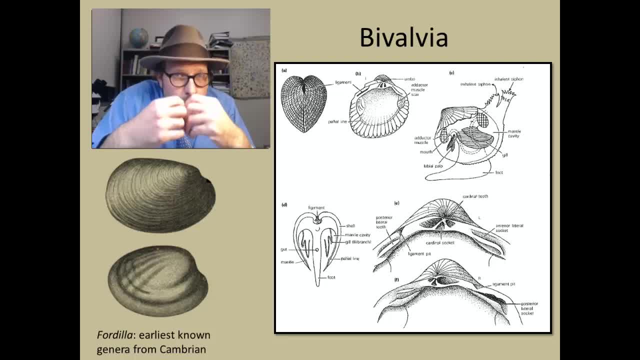 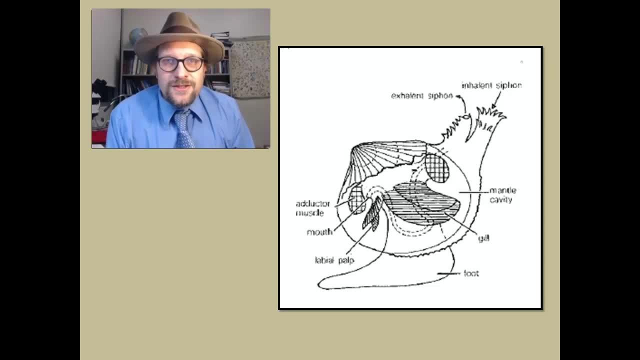 The ligament offers a soft hinge in which the shells can spring open like a rubber band. Bivalves have a fleshy foot and extend a siphon out of the shell. Bivalves can make a living by siphoning in detritus and food into the mantle cavity. 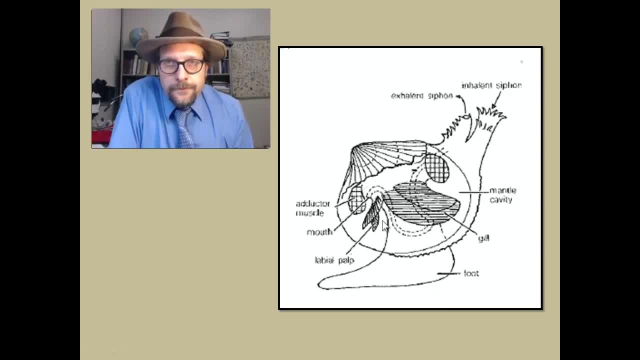 and they can be found in a series of labial palps into a mouth. Paired gills also hang out in the mantle cavity. in the rushing incoming water. This provides lots of oxygen to the shelled organism. The exhalant siphon expels the waste out of a separate opening for the anus. 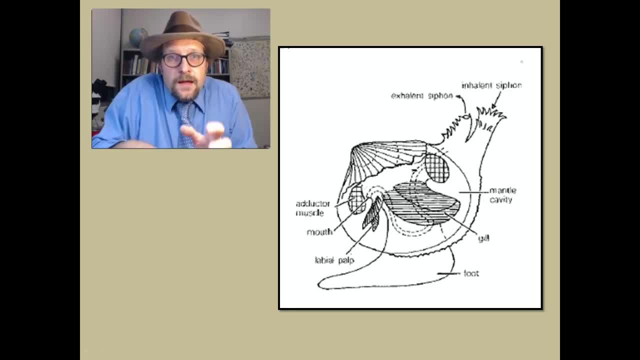 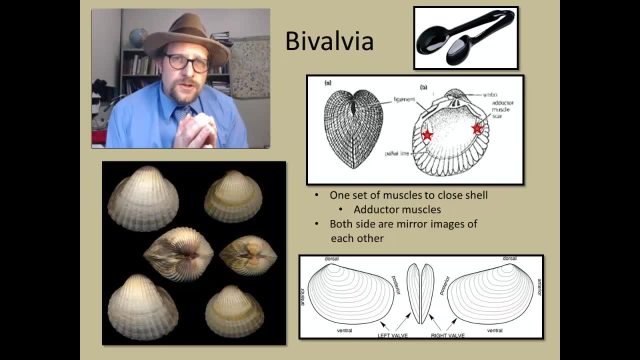 Bivalves are mobile. They can use food, They can shoot Foot And can quickly dig into sediment to escape predators or dig through the mud and muck. Bivalves close their shells by the constriction of a set of adductor muscles or a single. 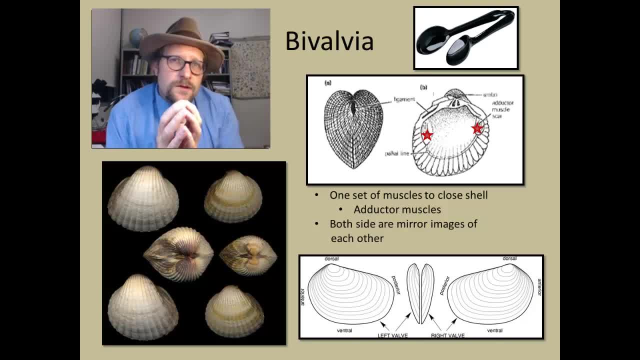 adductor muscle. in some groups These muscles close the shell. When relaxed, they open the shell. Hence bivalves lack a muscle to open the shells. and when cooked they open the shells to expose the mantle. Both sides of the shell are mirrored images of each other, with a hinge along the ligament. 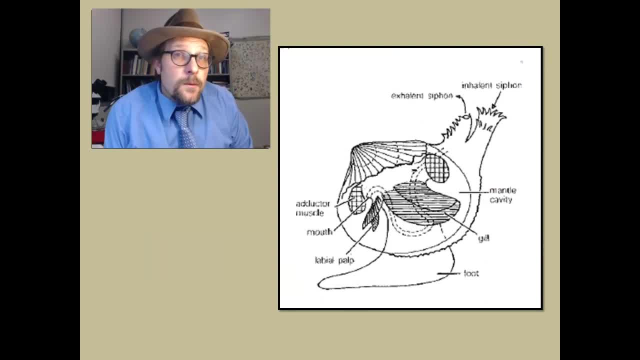 line that connects the two halves of the shell. One of the most remarkable things about bivalves is that they have a long foot and siphons that extend pretty far outside of the shell, which are only preserved in the fossil record as trace fossils. 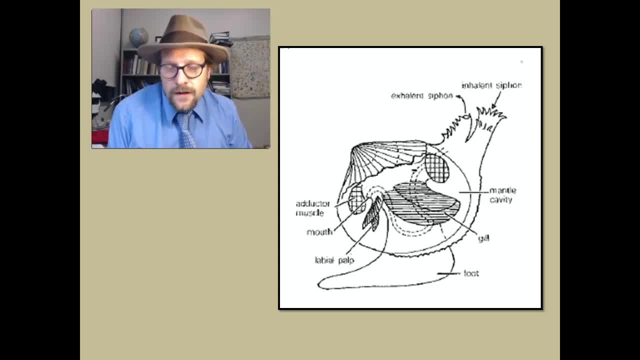 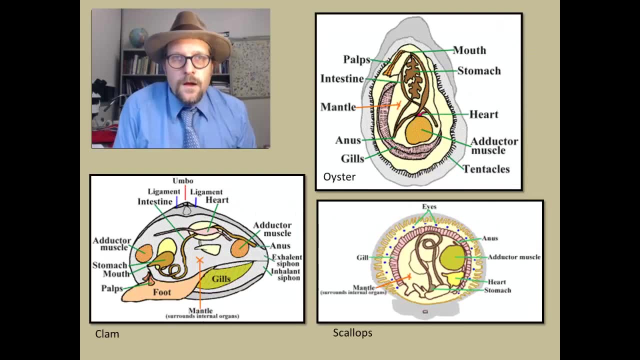 In fact, the movements of bivalves moving around in soft sediments is extremely common, but not always recognized by geologists in the rocks. So let's look at the anatomy of three bivalves that you are probably most familiar with, the ones we eat: oysters, clams and scallops. 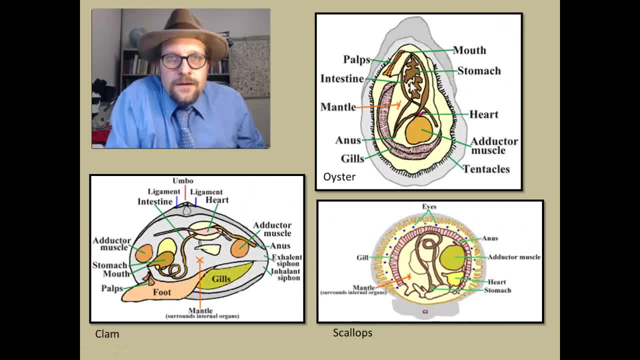 Note that in each of these groups it has a gut with a stomach, a mouth and an anus. The mantle is ringed by a set of gills. In clams there is a fleshy foot that comes out. This is often the chewy part of clams when you eat them. 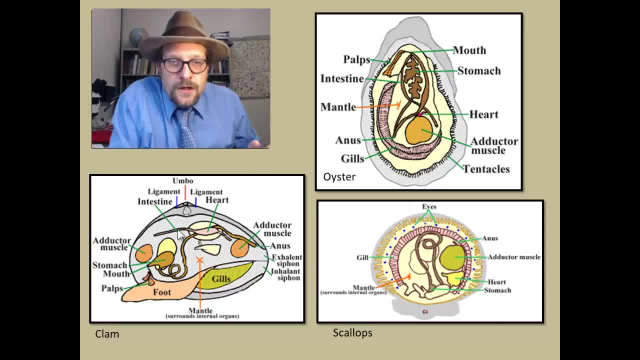 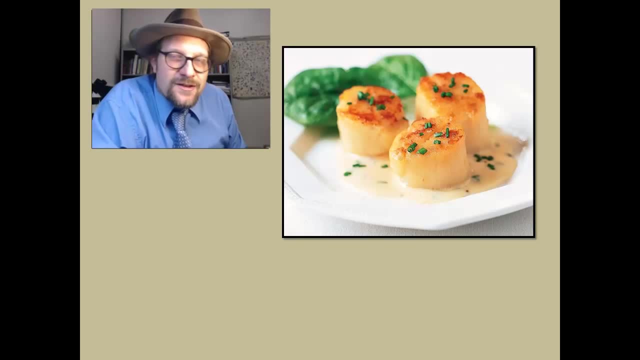 In all three groups there is a set of muscles that close the shell: the adductor muscles. These adductor muscles are rich in protein and they compose the meat of the shellfish With scallops. the adductor muscles are the portion of the scallops that you eat often. 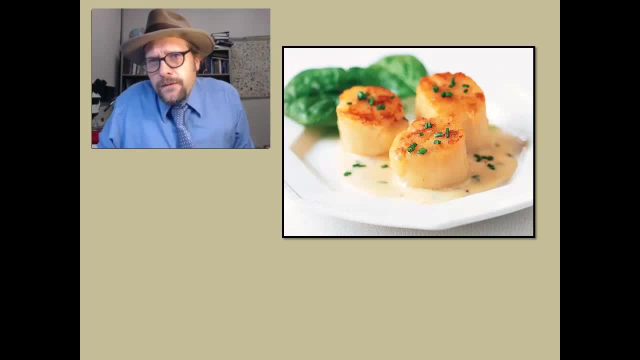 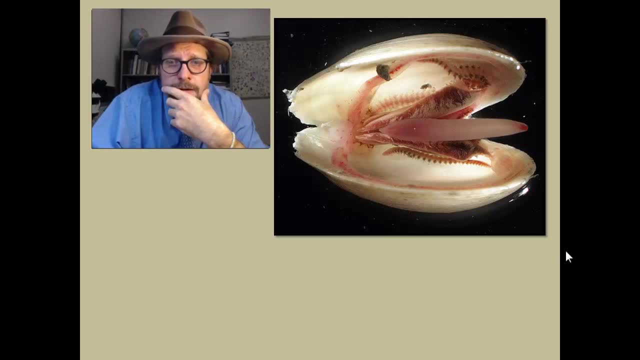 baked or fried. so the next time you cook up some bivalves, think about what you are eating. When you crack open a bivalve, you will find the fleshy foot, two sets of gills and filtering polyps that narrow down to a mouth with a gut tube that goes through. 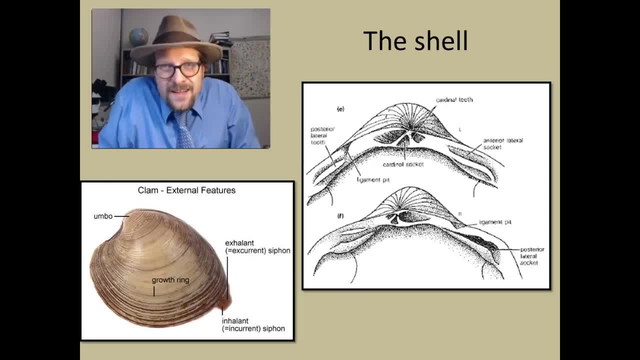 The shell is the part that fossilizes among bivalves and, as such, it is the part of the animal that paleontologists are most familiar with. The articulating, hinged surface contains cardinal sockets and teeth with broad pits. The shell is the part that fossilizes among bivalves and, as such, it is the part of the. 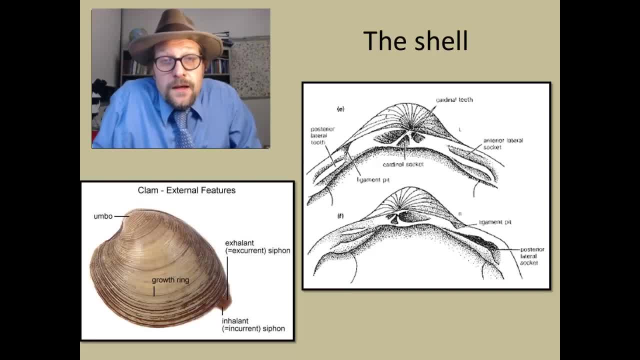 animal that paleontologists are most familiar with. The articulating hinged surface contains cardinal sockets and teeth with broad pits. These hinged lines can be an important feature in identifying groups in the fossil record. The shell also exhibits growth rings, which can be tidal or seasonal, and the umbo is 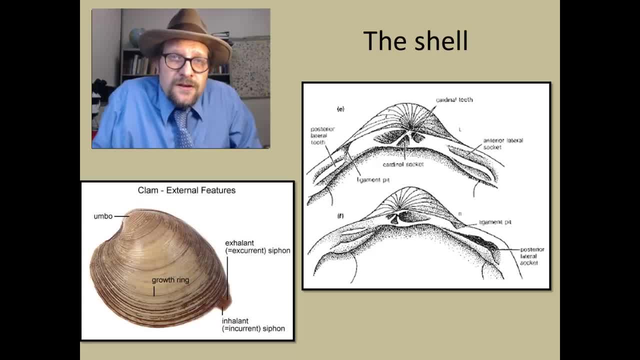 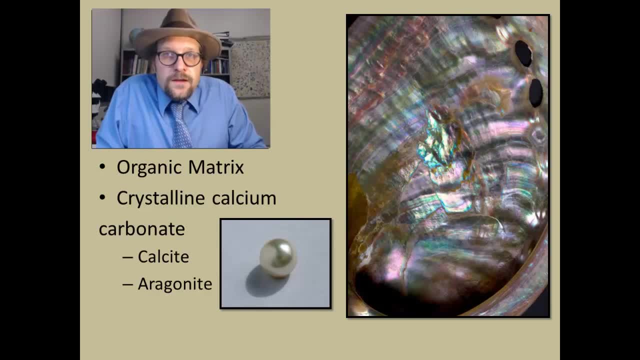 the initial growth protuberance on the shell, with one on each side of the shells. What are bivalve shells made out of? They are composed out of layers of crystalline calcium carbonate with an organic matrix. Unlike brachiopods, bivalves make up the bivalve shell. 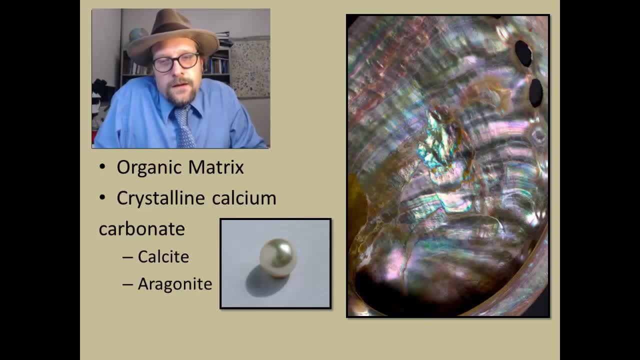 Bivalves make a shell with both calcite and aragonite. Both calcite and aragonite are calcium carbonate, but with different crystal lattice structures. Aragonite is unique in that crystals form needle-like projections which diffract the light and produce iridescent shades of different wavelengths. 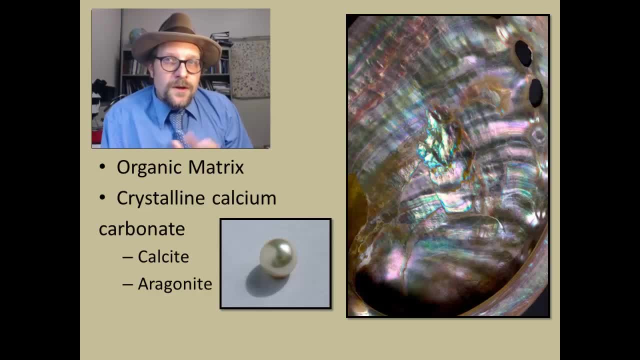 That effect is often called the mother-of-pearl and is one of the reasons that pearls are so shiny. These arachnidic crystals are fragile and with burial heat and pressure they are quickly replaced with calcite in fossils, although sometimes original aragonite can survive the 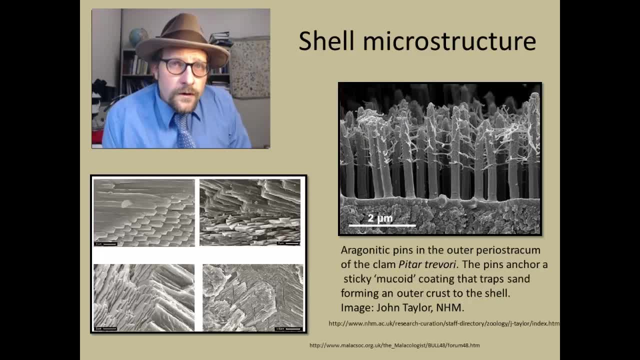 destructive effects of fossilization. Here are some wonderful SEM microscope images of the arachnidic crystal surface of the outer perioscium of the clam Pithar Traviae. These are arachnidic crystals. They can trap stiches. 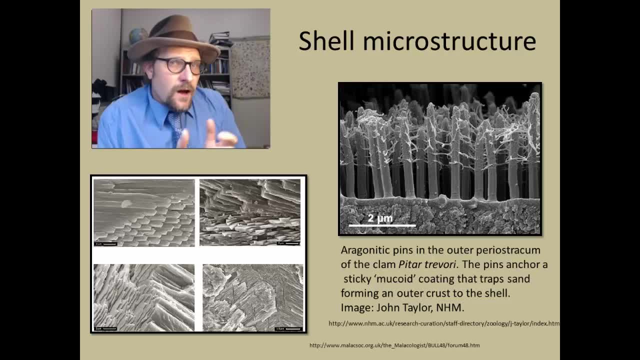 They can trap stiches. They can trap stiches. They can plant stiches. They can caught stiches. You can take a piece of scarniaURünden and insert it into a piece of calling cloudourden. 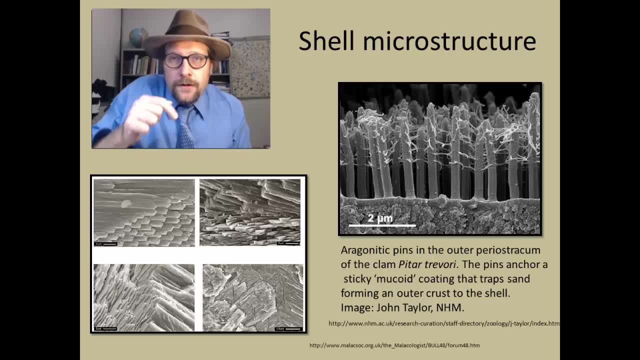 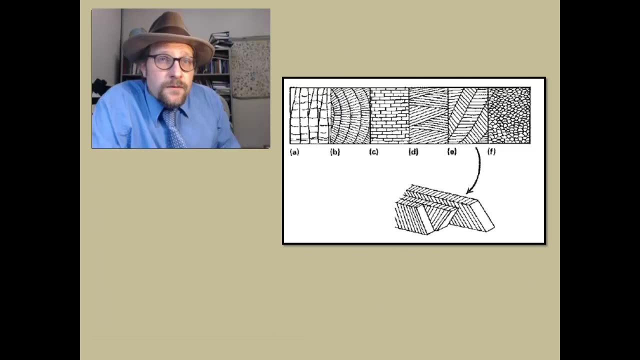 right here. They can antiproteinize theirucks by蘭 wraparodii, about 20-30 percent of Aries ב�reatur and teuxine around it up to 30%. They can also attract the yselectrinus, being rich in broncholite as it has Tellurideazole号, which is ałoacynide. 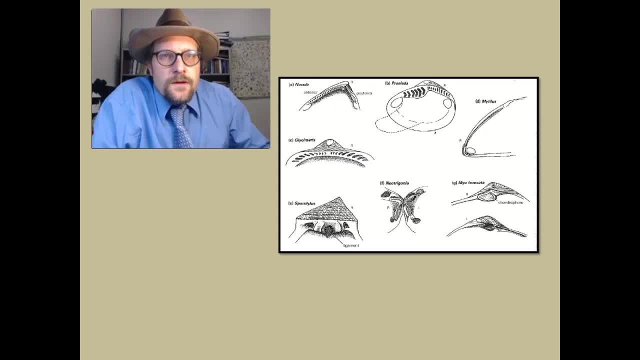 that is packed into the energy of the добав186.. Now, of course, they can also bind used-to-die provenantly offầ�enц Mus record. The hinges of the shells are the most important component of the fossil shell and often paleontologists 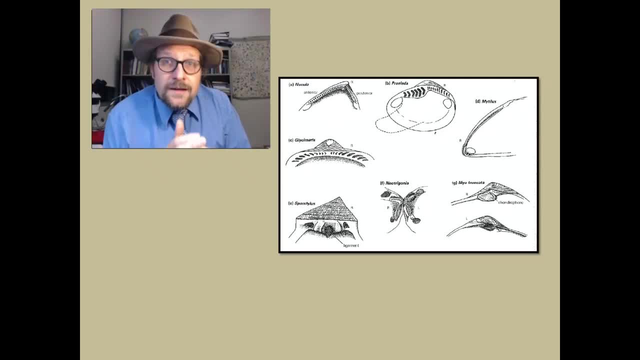 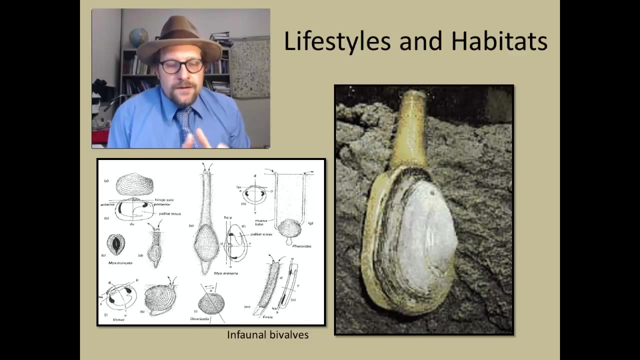 seek out specimens that preserve these hinges, since their anatomy is unique to species in general. Hence, when only fragments of the shell are preserved, it is often the hinge that is most important for identification. Most bivalves are infaunal. that means they live buried in sediment. 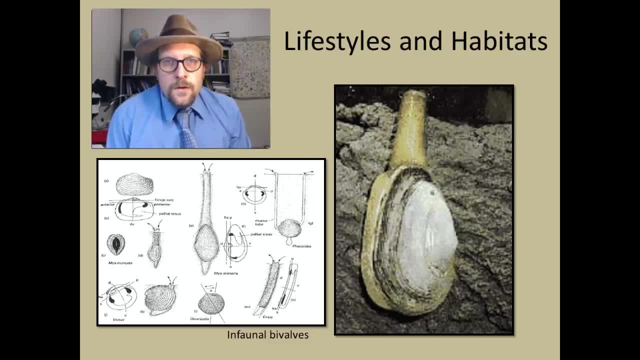 The only connection to the surface waters is a long siphon that includes a path for incoming water, for filtering, for food and oxygen and an exhaust siphon to get rid of waste. The siphon can be very long in some forms. 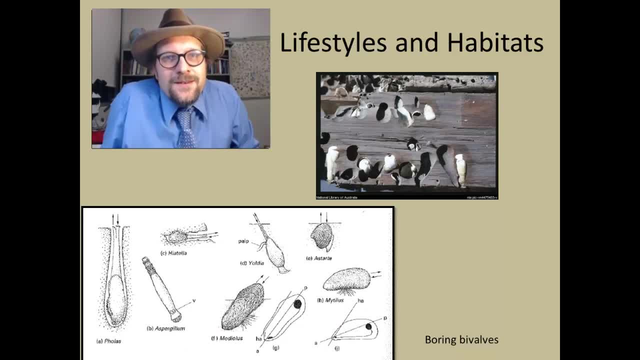 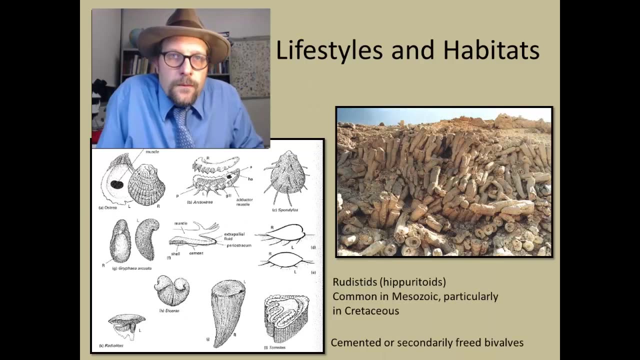 Other bivalves can be burrowing bivalves. They can use their foot pedicle to burrow down or burrow into hard substrates like wood and hard rocks. This burrowing can add additional water. One of the most unusual groups of bivalves are the Rudistids, a group common to the Cretaceous. 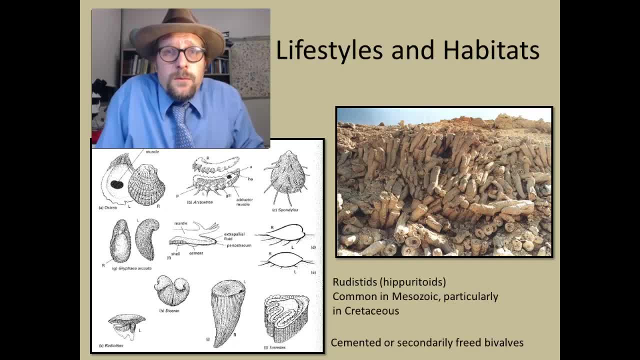 which form reefs. These colonial bivalves form long tubes capped by an upper shell and a long tubular-like lower shell. They are particularly common in the Cretaceous in Europe and North Africa. Not all bivalves are sessile. 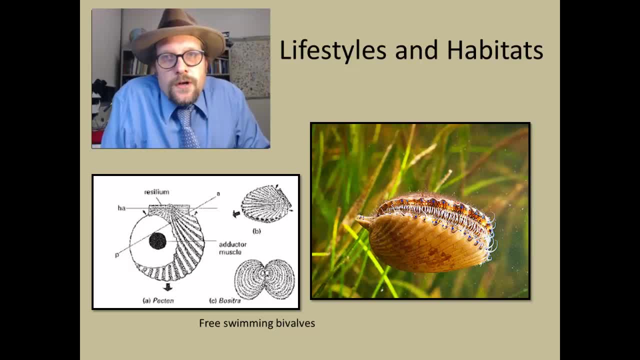 Scallops are mobile and free swimming. They use the two shells. They propel themselves through the water column and can move about on the ocean floor. They have a long row of eyes that can help them see where they are going. Other mollusks also develop eyes and light-sensing organs, which are needed when animals become. 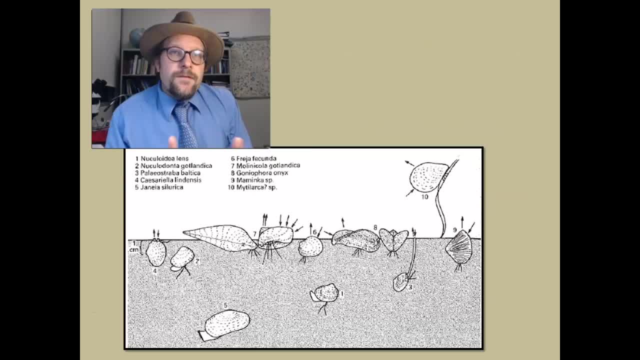 mobile and need to see where they are going. Bivalves occupy a huge range of habitats, including freshwater systems. All bivalves are aquatic. I'll see what the next slide shows. You can see with the next class of mollusks that there are some mollusks that made the 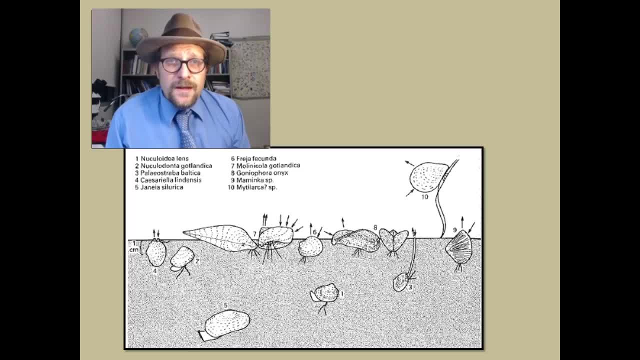 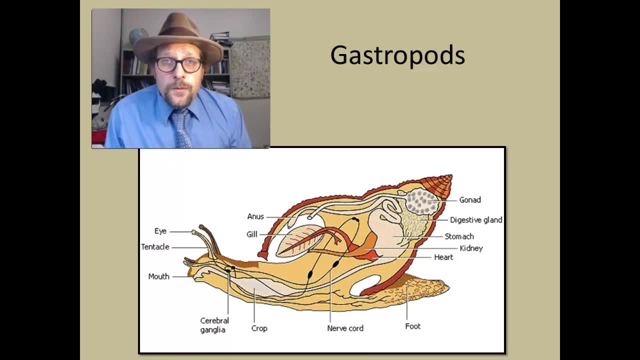 transition to living on land. These are the Gastropods, the snails. The Gastropoda is the first group of mollusks that have a head. This is a really important innovation, since it also leads to the placement of sense organs. 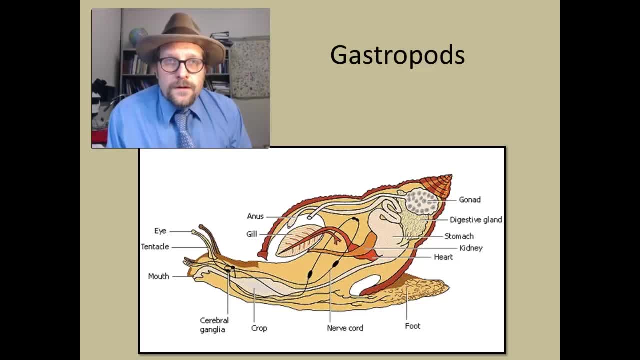 such as eyes, in the front of the animal. These sense organs then move to the front of the animal. These sense organs then move to the back of the animal. These sense organs then move to the front of the animal. The head and the foot can transport information to the rest of the body along nerve cells. 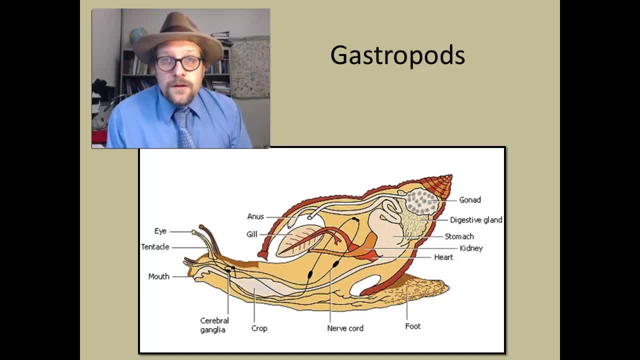 that can trigger movements in the foot and mucous glands that are used to move the gastropod or snail forward across the surface. The head and foot can be retracted into the coiled shell, with the foot closing off the wall. The gastropods have to have muscles to pull these organs into the shell. 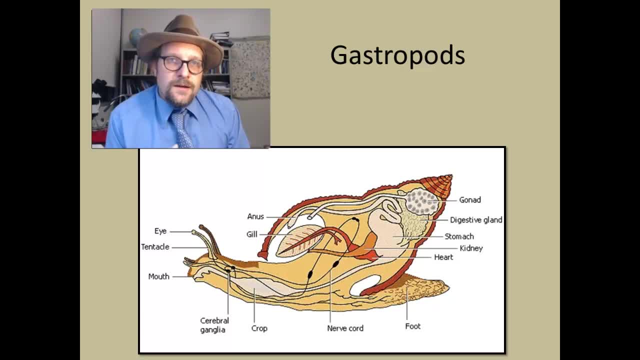 The gut, digestive organs and gonads are located deep in the shell and allow for retraction of the head and foot. Many gastropods are hermaphroditic, although some can be male and some female, with sexual reproduction that can be done by bizarre darts that males can shoot into females. 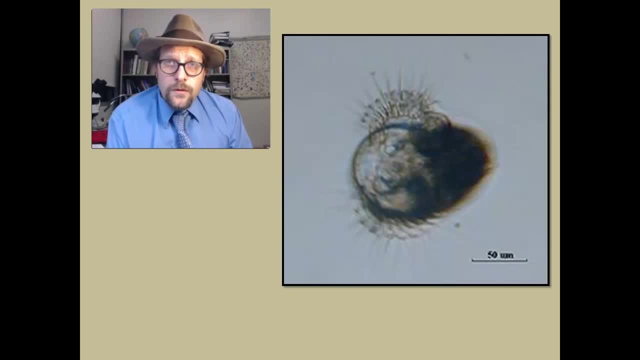 Snails lay eggs which hatch into larvae known as trochophores that look like worms. This worm-like larvae quickly develops into a sail-like vellum that has ciliated cells that help the fellow navigate and propel through the water. During this stage, the gastropod twists and begins to grow a twisting shell, while the 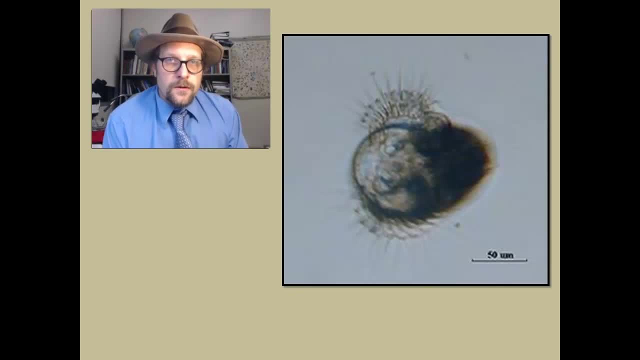 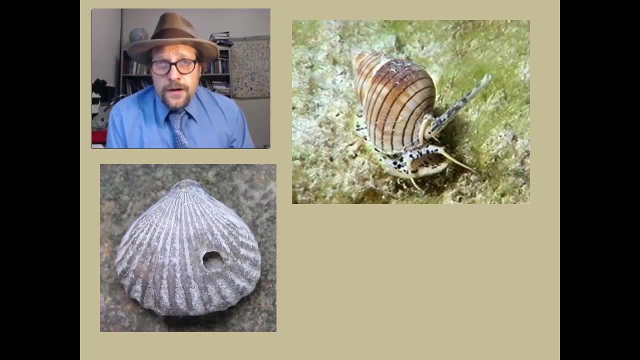 vellum forms the foot of the developing early little snail. Once it reaches this stage, it can use the muscles and mucosal glands for movement on the surface. Gastropods are predators and can bore into other organisms. They can be herbivores, where they graze on algae, and scavengers, feeding on dead things. 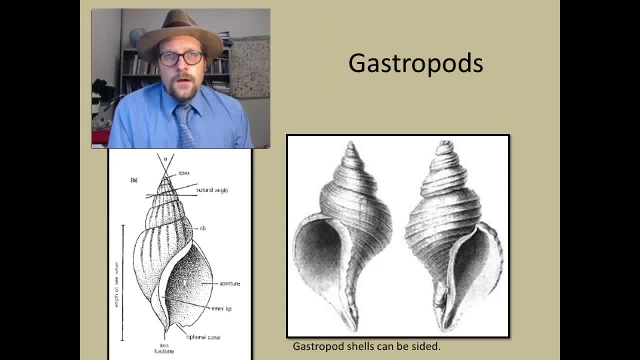 that accumulate on the floor of the ocean. The twist in the shell gives gastropods a unique morphology that can vary in hundreds of different ways. One of the simplest ways to identify a gastropod is by looking at their body shape. The most common morphological features are the direction of the twist, as in dextral. 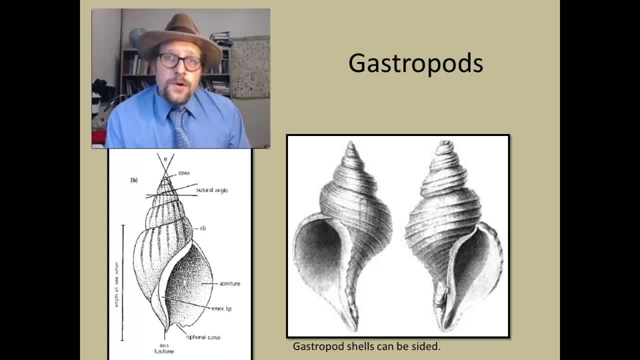 to the right or sistral to the left, producing mirrored images of shells in different forms. The pointy end of the shell is called the apex. The coil angle is the schutert angle. Many forms have ribs that run the length of the shell. 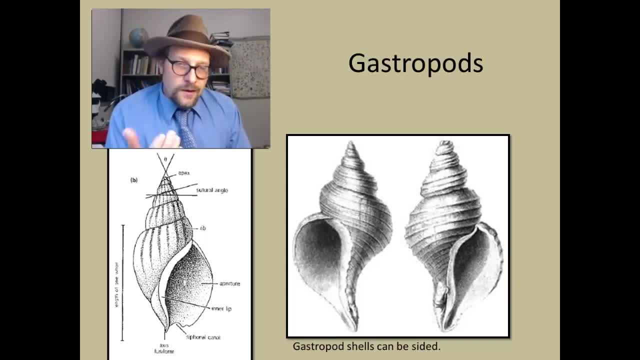 The opening is called the aperture and has a flexed inner lip on one side. The upper lip of the shell, which is the second lip, is a selenium with a puncture. on the left side, The cleft lip is a limpid lip and is the cause of the large, very thin, jagged teeth. 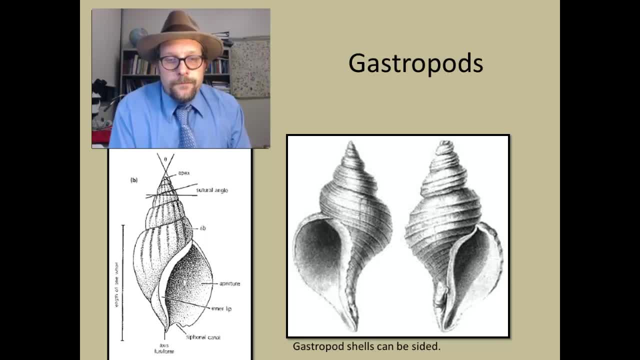 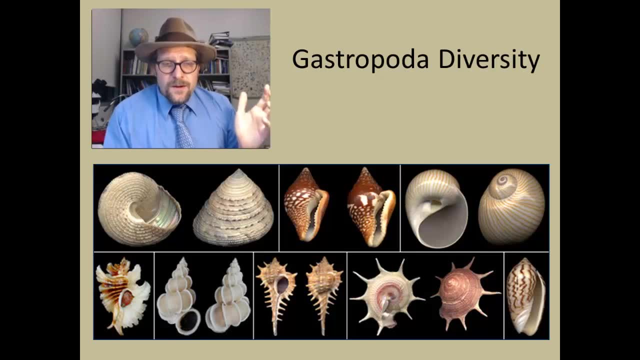 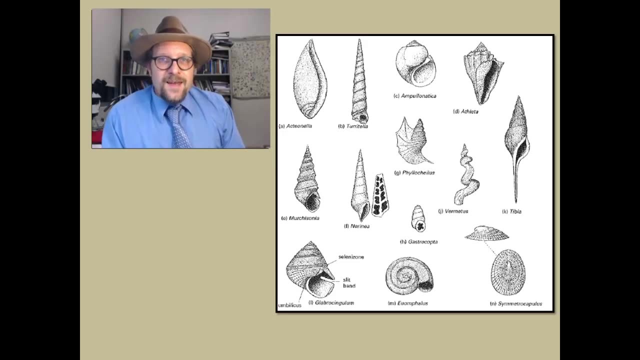 Often there is a groove for the siphon called the siphonal canal. Gastropods are very diverse and need a class all of their own, because they are fascinating and we just don't have enough time to cover all of them. Many different forms of gastropods exist and because their shells readily fossilize, we 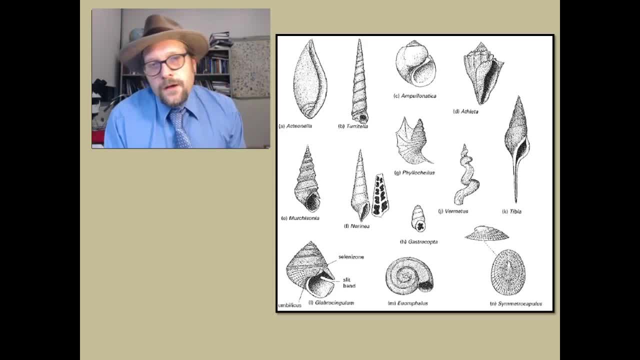 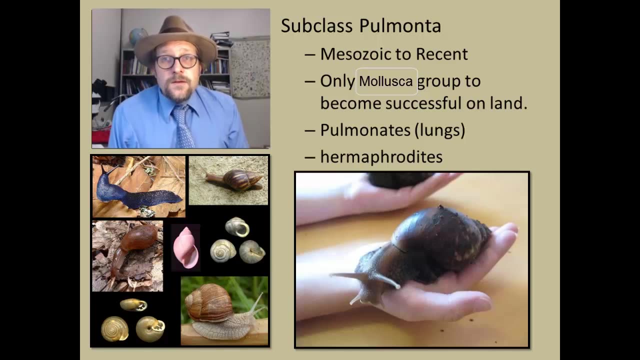 can identify them down to species. They are amazing for reconstructing the ancient environment in the past because many of them are found living today that we find in the fossil record. I am going to highlight only one group of gastropods, the subclass pulmonaut. 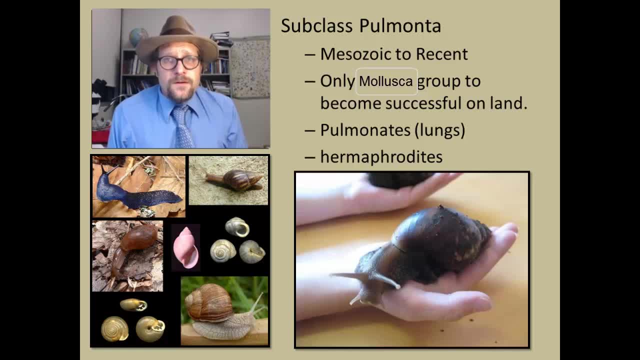 These are the group of gastropods that you are probably most likely familiar with, since they made the leap to living on land. They are known from the Mesozoic to recent, and instead of gills, they have developed lungs. These lungs allow them to breathe on land, although they are still connected to the water. 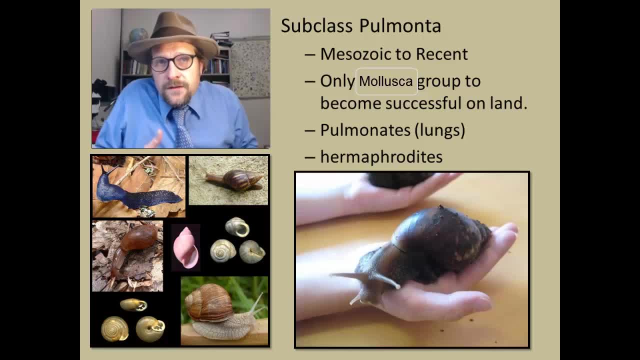 for reproduction. Most are hermaphroditic, which means that each individual has the ability to start large colonies of gastropods. So just one little larvae gastropod can make it into a pond or new environment and it can breed with itself to produce hundreds of new babies and establish a new population. 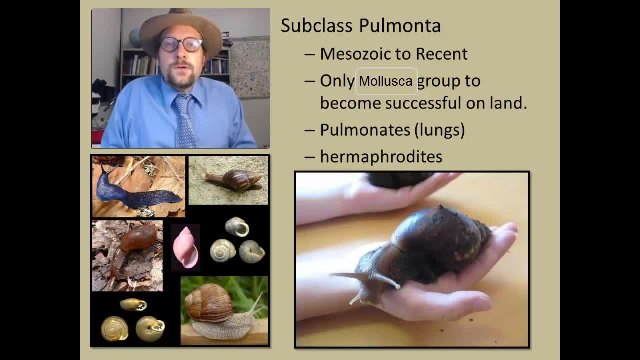 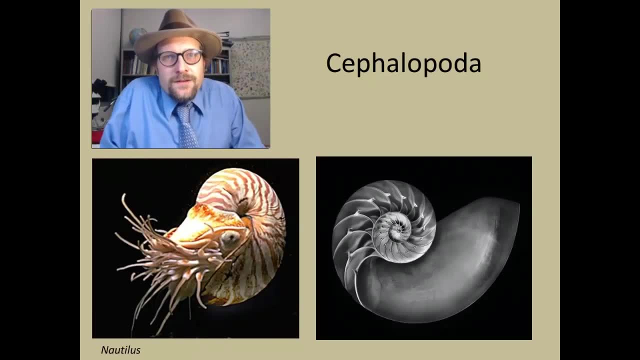 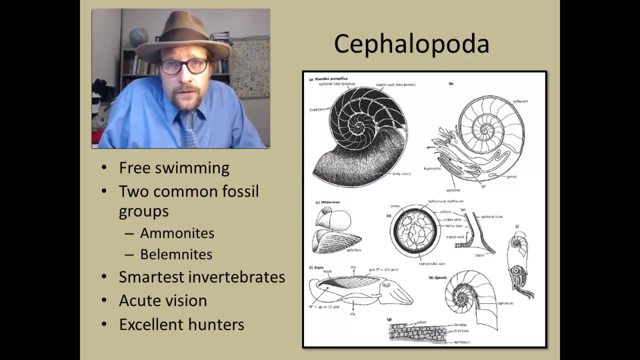 In the fossil record. this means that you can find large numbers of individuals deposited during these big population births. Now let's look at the last group of mollusks, The highly successful cephalopoda. This group is only found in marine waters and includes the modern nautilus, the agronauts. 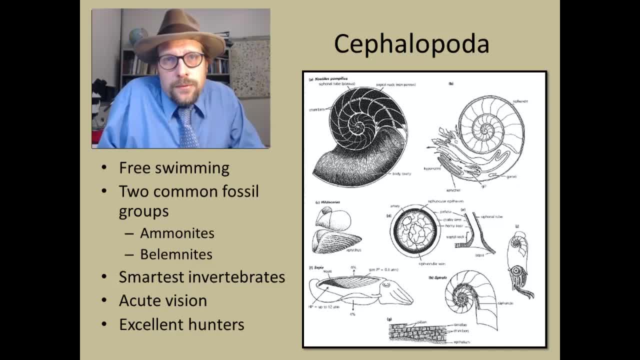 squids, octopuses and the extinct ammonites and blemonites. Cephalopods have the most well developed heads, including the development of a brain, a nervous system and complex sensory organs such as eyes. These are the most intelligent of the invertebrate groups and likely develop these complex brain. 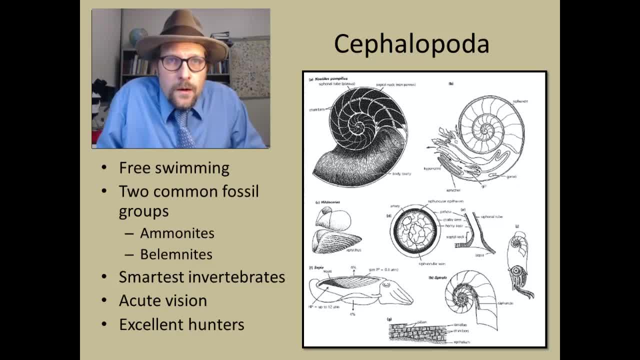 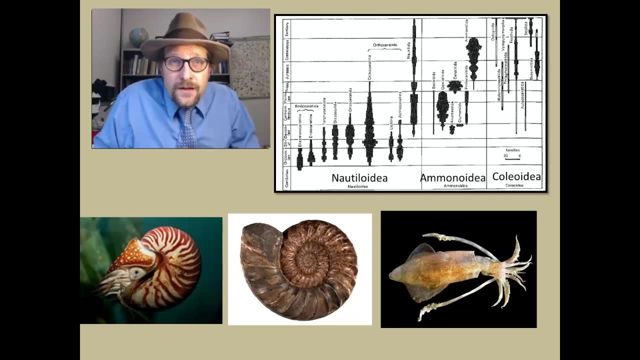 organs from the shared feature of having extreme mobility, which means that they must process information quickly from the environment to survive. Cephalopods are swimming carnivores and feed on larger prey. Cephalopods are divided into three groups: the Nautiloidae with a fossil record from. 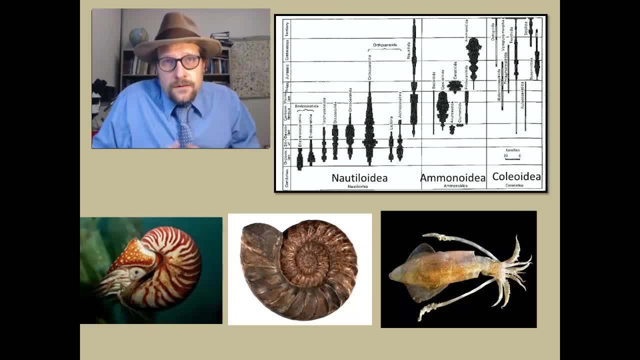 the late Cambrian to the recent, the Ammonitae from the late Devonian to the late Cretaceous, and going extinct at the end of the Mesozoic, with the dinosaurs And the internal shell or shell-less Cholindidae known from the Carboniferous to recent, which 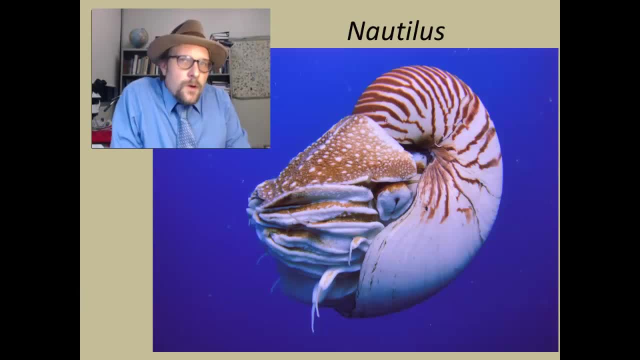 includes octopuses and squids. The Nautilus is the only living genus with a coiled external shell which is much better represented in the fossil record and much more diverse than the single genus we have living today. The living Nautilus does give us some insight into how these coiled cephalopods of the past 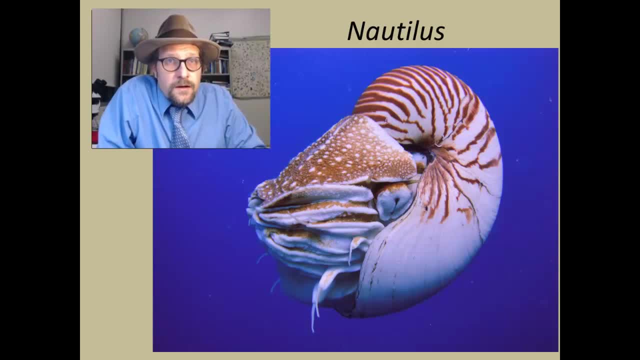 may have lived. The Nautilus lives in a shell that is divided into chambers or cambria. These are separated by septa that concave in much like the aperture. As the animal grows, it generates a new chamber, coiling the chambers over time to make that. 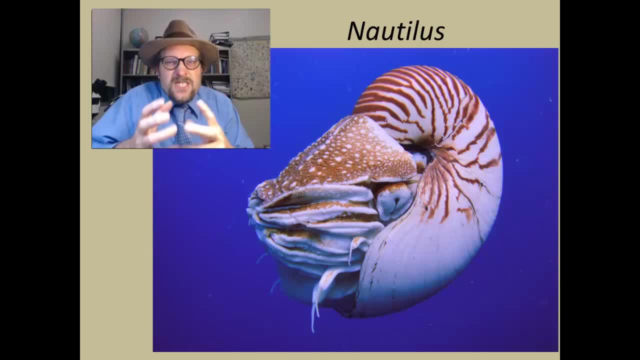 coil. The biggest chamber is the body chamber, where most of the fleshy part of the animal is found. The chambers are connected by a canal called a sphyncloncle, which allows the animal to adjust its buoyancy of the shell by extracting fluid and leaving it to be air-filled. 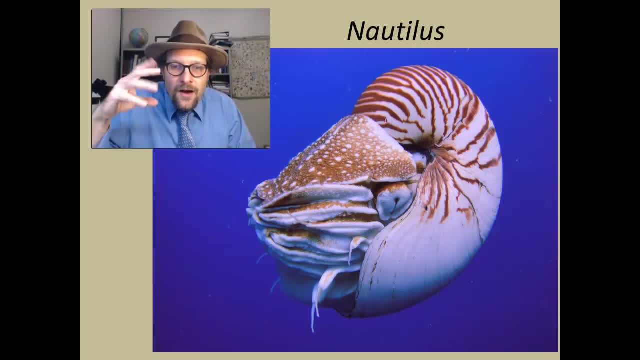 The Nautilus also has two eyes on either side and long tentacles that are used for capturing food and sexual mating. As a very mobile nektetic organism, the Nautilus uses a water jet to push itself through the water and escape predators. 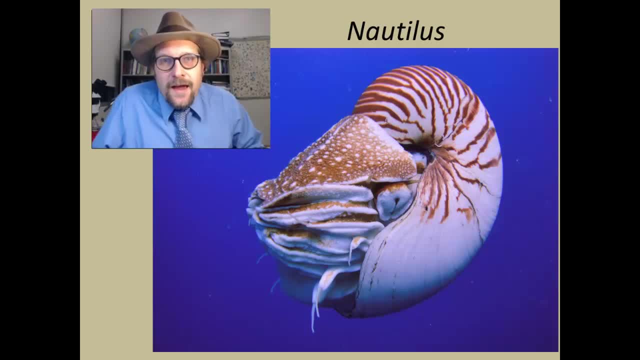 It can also cloud the water with ink using an ink sack. The Nautilus is a very mobile nektetic organism. The shell of the Nautilus is made of aragonite in two separate layers. Sometimes the original aragonite layer is preserved in the fossil record giving these 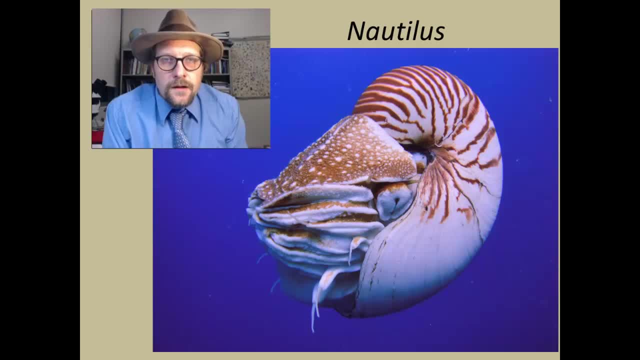 coiled fossils a pearly appearance. The shell of the Nautilus gives it an advantage to live in deeper depths of the ocean, living at depths below 75 meters in the dark waters below the photic zone. Nautilus can rise during the night and hunt the dark waters for prey. 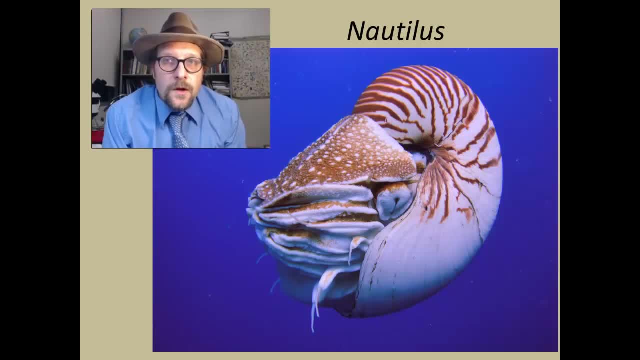 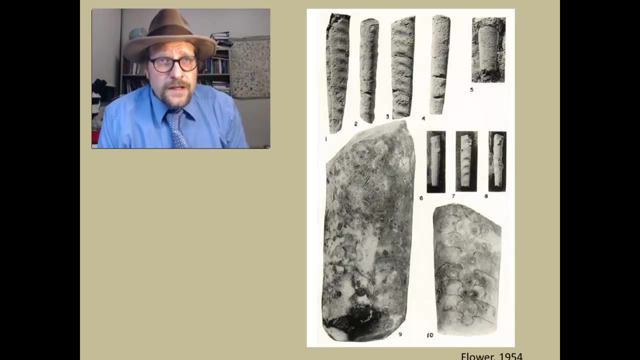 The Nautilus is a very mobile nektetic organism. They can then dive down to depths where larger fish and sharks can't follow. The shell allows them some protection from the increasing pressures of these deeper depths of the ocean. The oldest cephalopods are found in the late Cambrian, such as the rather straight shells. 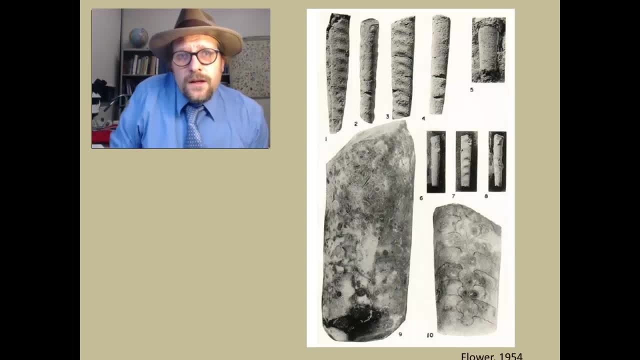 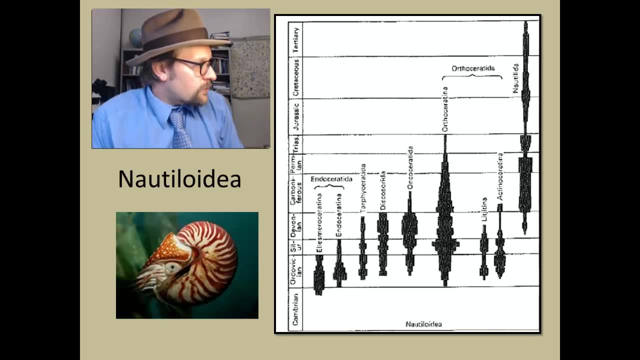 of the Placonoceros, But quickly afterward coiled cephalopods become very common and diverse. The Nautiloides were very common during the Ordovician to the Carthaginian period. The Nautilus is a very mobile nektetic organism. 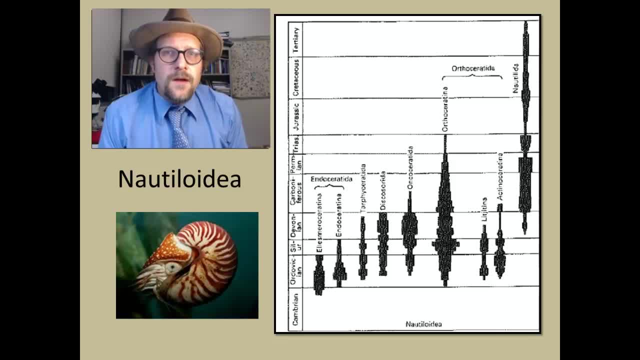 The Nautilus is a very mobile nektetic organism. The Nautilus is a very mobile nektetic organism Since the Mezzanine Nautilus is common in the Mithraidae and Necromancer and is also a common nektetic organism. 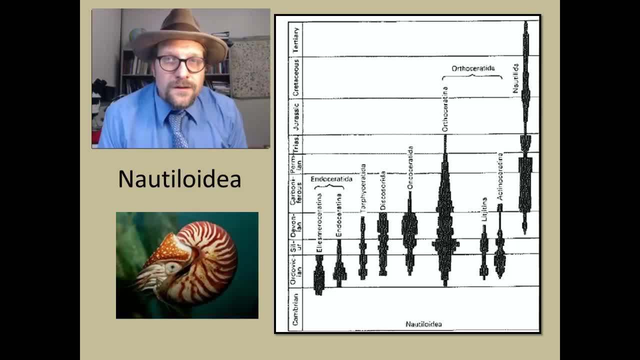 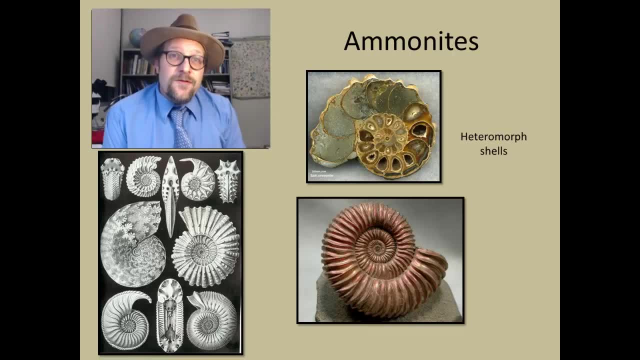 Today, Nautilus is a small remnant of this once very diverse group. The ammonites are probably the most famous of the marine fossil invertebrate groups. They first appeared during the Devonian and survived until the end of the Mesozoic going. 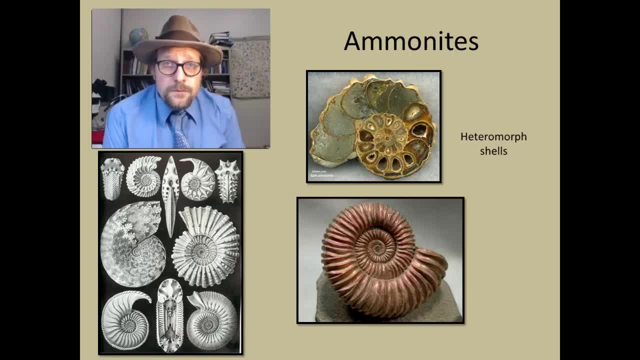 extinct with the dinosaurs. They are common fossils and popular with both amateur paleontologists and biostratigraphers. Ammonites are heteromorphs in which the shell can be seen quite이트, like this. Ammonites are heteromorphs in which the shell can be seen quitehte, like this. 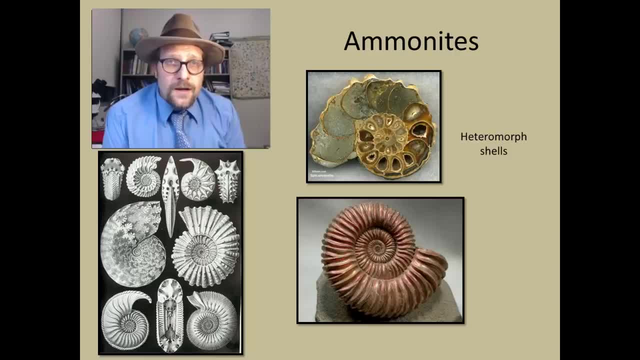 These are common fossils and popular with both amateur paleontologists and biostratigraphers. seen coiled on the sides of the shell, where in nautiloids the coils cover the smaller inner coils, This difference in coiling is thought to be from a separate origin of coiling from two. 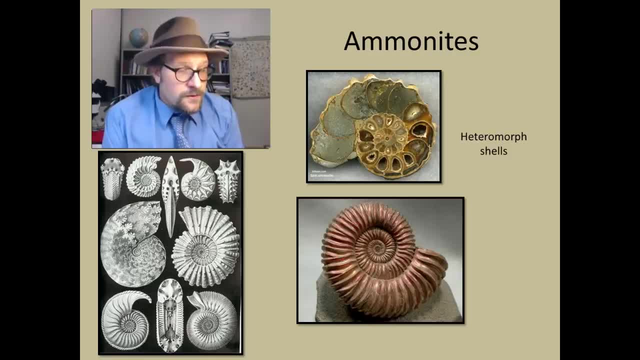 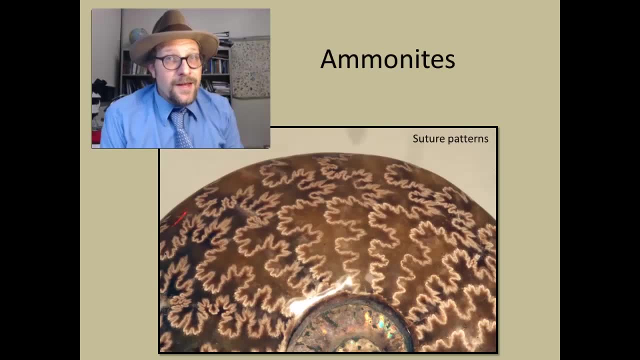 different early uncoiled cephalopods and hence the coiling found in the two groups is convergent. Anyone interested in ammonites must learn the complexities of recognizing the suture morphology, which is key to the identification of different species of ammonites. 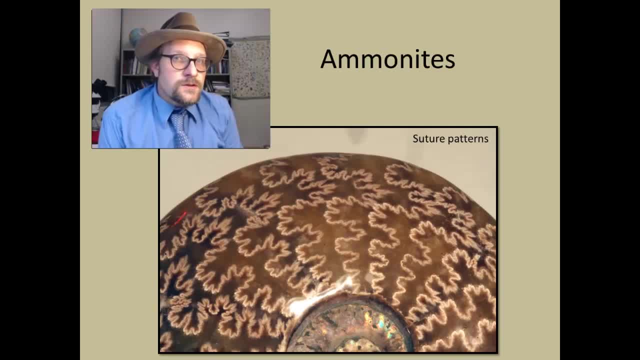 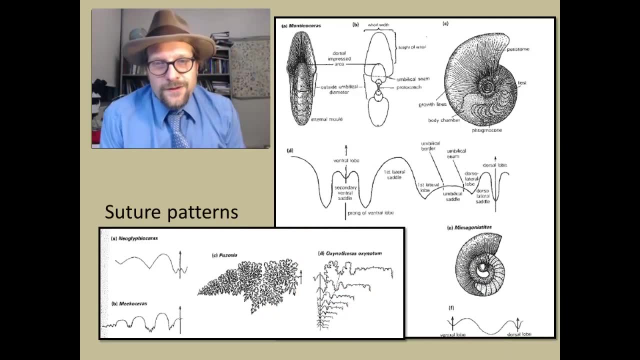 Ammonites have complex suture lines in their shells. These mark the junctions between septum. They can be seen even in fragmentary fossils. Suture morphology is often illustrated with unique terms for the various waggles of the suture line. 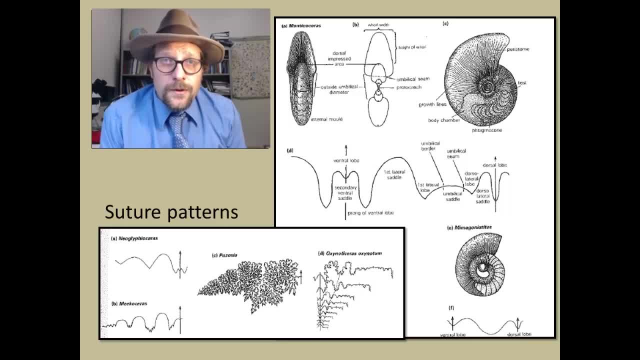 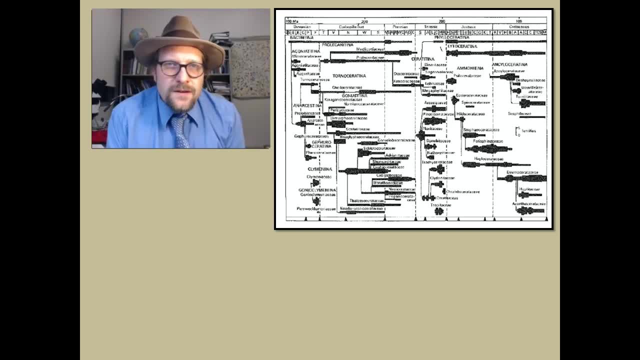 Some are extremely complex, while others are rather simple. Ammonites are amazingly diverse, with hundreds of groups represented in the rock record. Because there are so many species and they are easily recognized from sutures and they have short durations in the fossil record, they are excellent index fossils particularly. 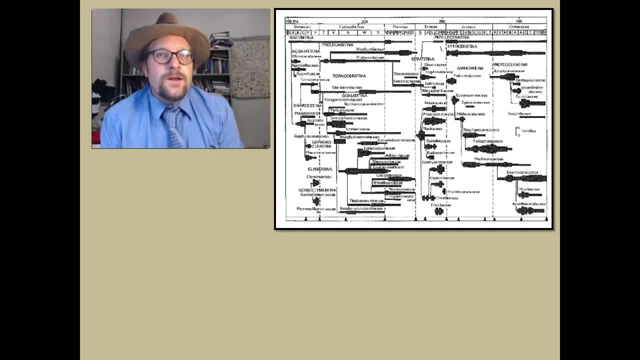 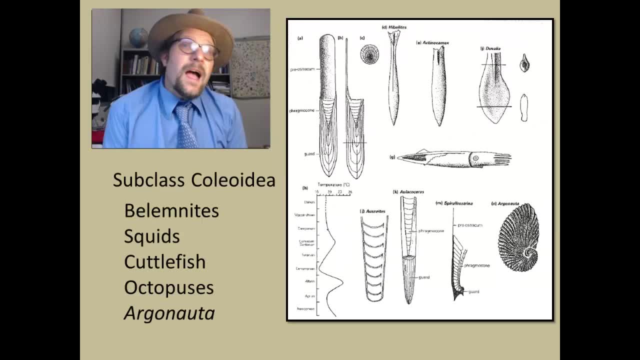 during the Devonian to Cretaceous. Here in North America, the ammonites are an important index fossil for the western interior seaways during the Jurassic and Cretaceous periods. The last group we will examine is the subclass Colneidae. 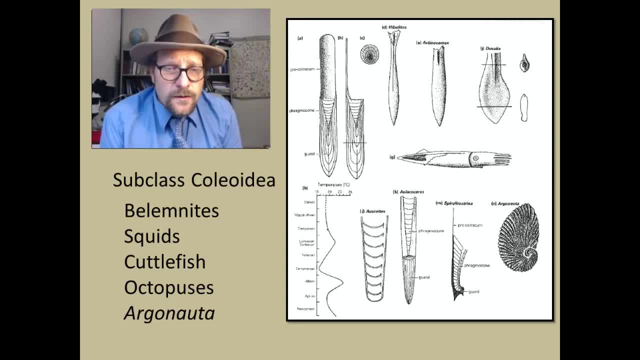 That includes the Blemenites, The squids, the cuttlefish, the octopuses and the Argonauts. These are recognized in the fossil record by several members of this group having an interior skeleton and calcite forming the hard part that is preserved in the fossil. 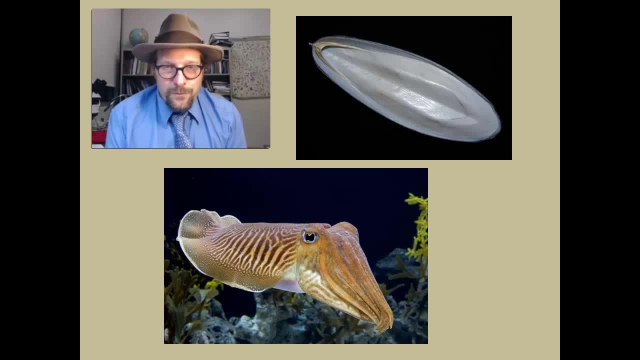 record In cuttlefish. this is a calcareous bone that helps with buoyancy. This can be preserved in the fossil record, since it is composed of calcium carbonate. This chemistry is also why it is given the name. It is also known as the Cretaceous. 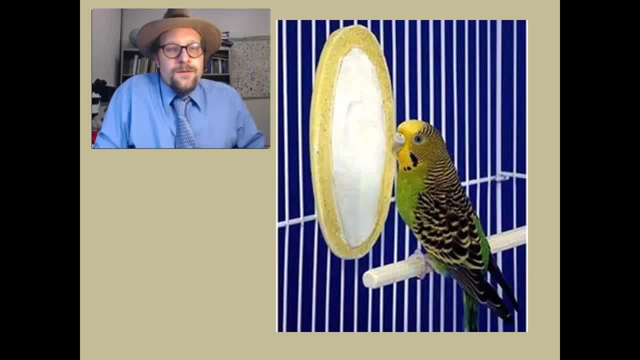 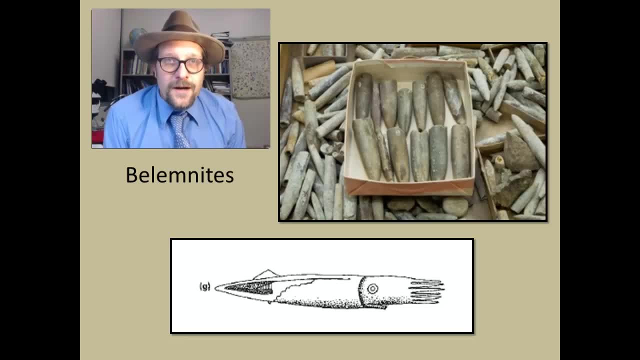 This is why it is given to birds and sold in pet stores as a source of calcium. The Blemenites are another group that have a hard part that is preserved in the fossil record, but the group is entirely extinct but probably likely was related to modern. 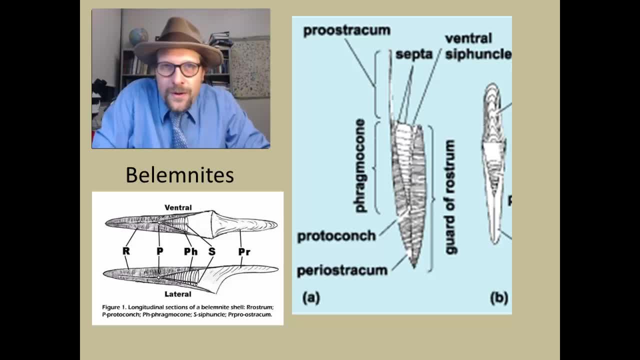 squid. The shell of the Blemenites is composed of three parts. The largest part is called the guard, a bullet-shaped cylinder of solid calcite. Further back is the Argonauts. This is a magnetic phragma cone, a cone-shaped structure. 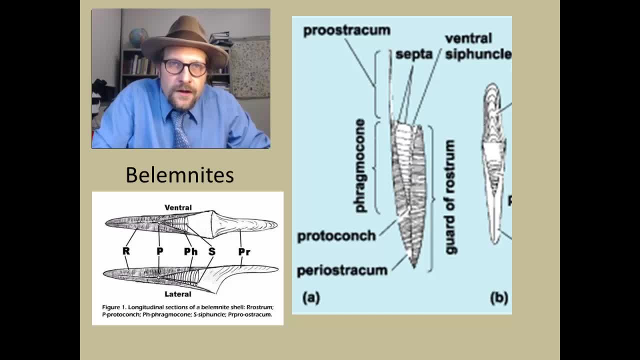 Then, further back, but very rarely preserved, is a prooscium, a flat, expanded tongue that actually would have covered some of the body of the squid-like creature. The guard is the part that most often preserves, and inside it is a narrow tube or opening. 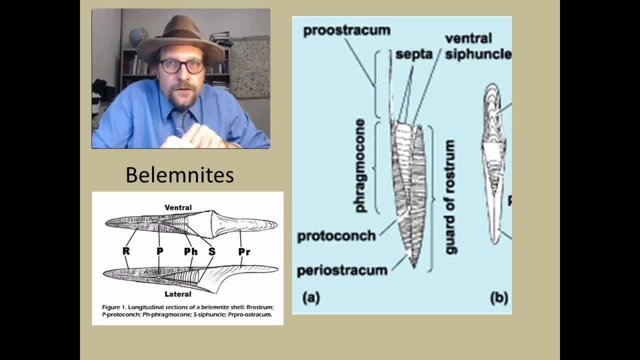 a channel that runs through the center. The guard is the part that most often preserves, and inside it is a narrow tube or opening a channel that runs through the center, Much like the coiled cephalopods. the guard is the part that most often preserves, and 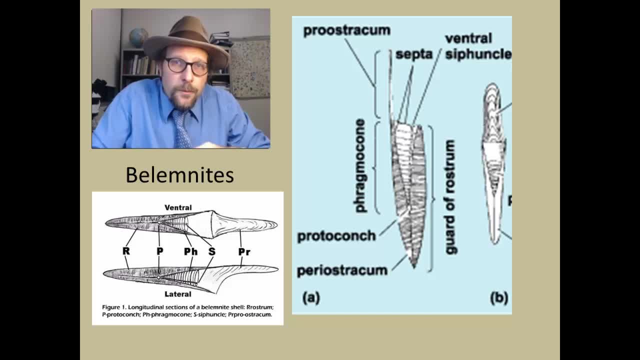 inside it is a narrow tube or opening a channel that runs through the center. The guard is the part that most often preserves, and inside it is a narrow tube or opening a channel that runs through the center. The guard is the part that most often preserves, and inside it is a narrow tube or opening. 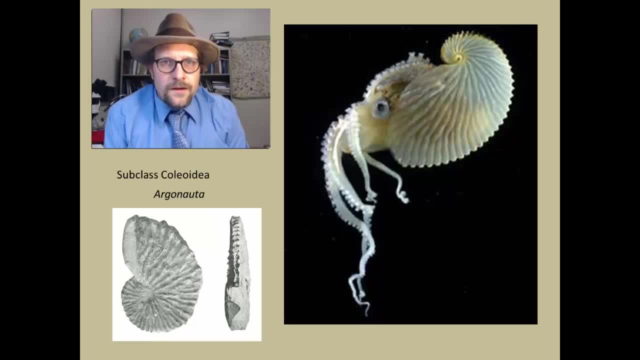 a tunnel that approaches the bottom appear at a certain POCKET. These should be real P норм paper nautiluses, and while they look like a nautilus or even an ammonite, they are actually the reproductive chambers of female octopuses.